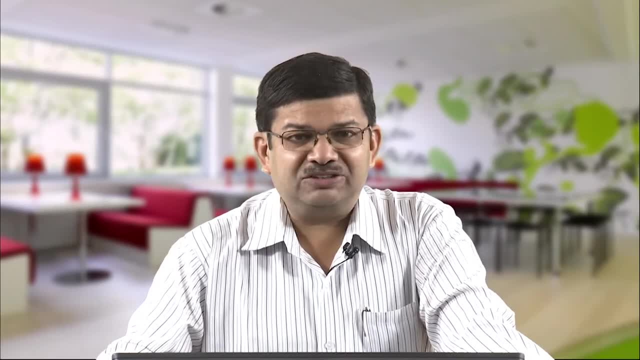 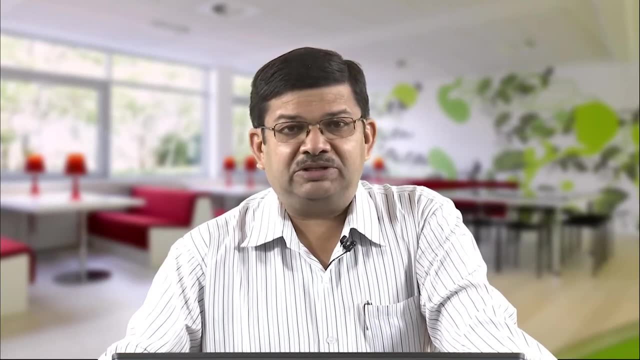 And if we see an image of an instrument, Let us see an image of a piano, and the piano is not too high. So this is because the piano is not too high, so it is not too low And thewirth of the piano is not too high. 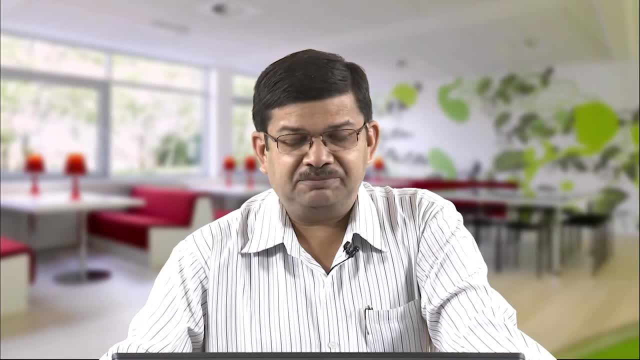 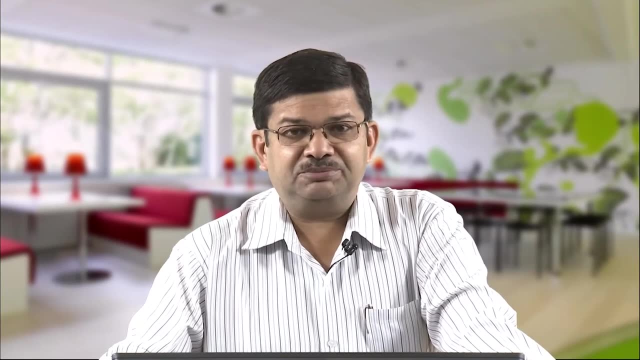 It is a quite low instrument, So the number of notes that is in the instrument is very, very low and therefore you cannot help but consider if it is enough. So this is the solution. So this is the solution. So let us continue. 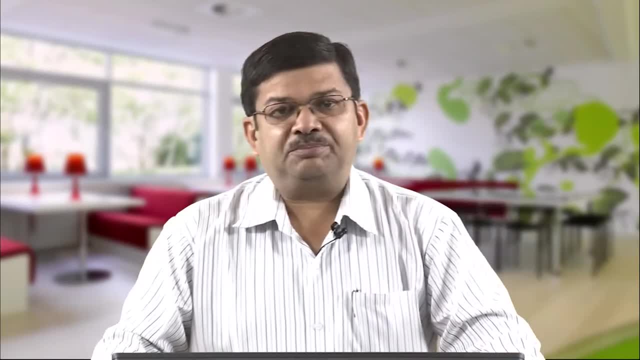 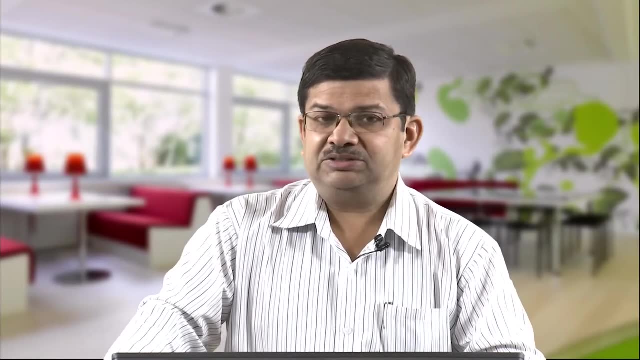 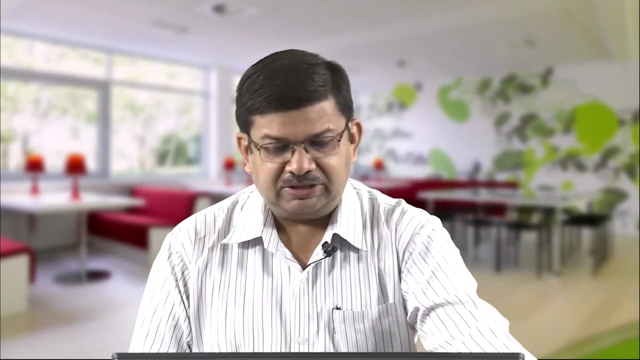 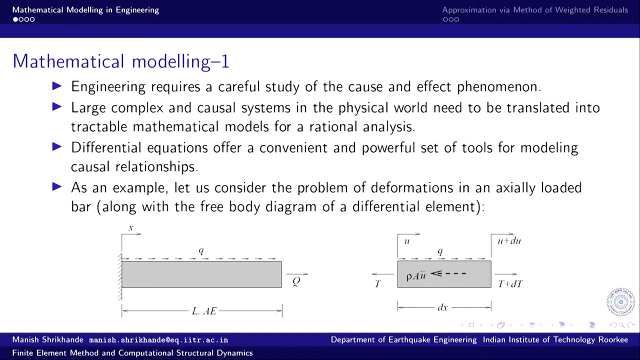 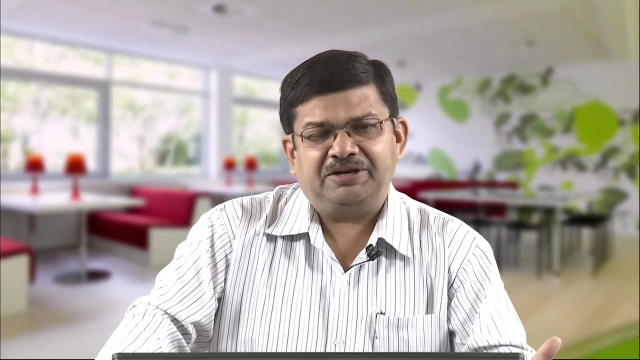 approximation, so that our purpose, I mean of coming up with good engineering designs and products- are adequately met. So to start with, the problem of the process of mathematical modeling is the first step of any engineering analysis And for any engineering analysis we need to. any kind of engineering requires a very 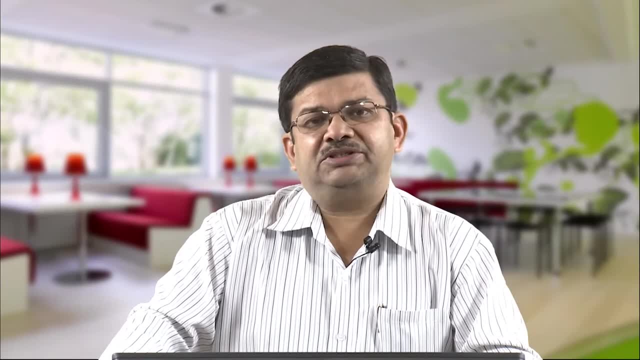 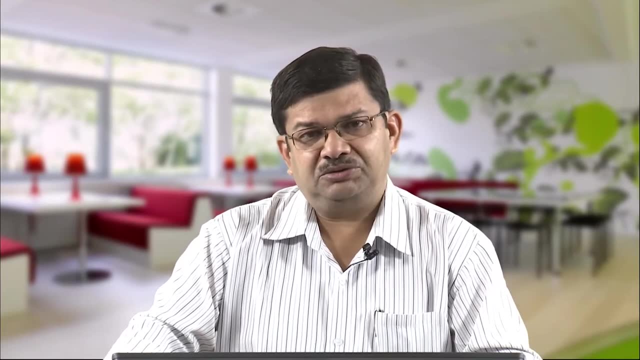 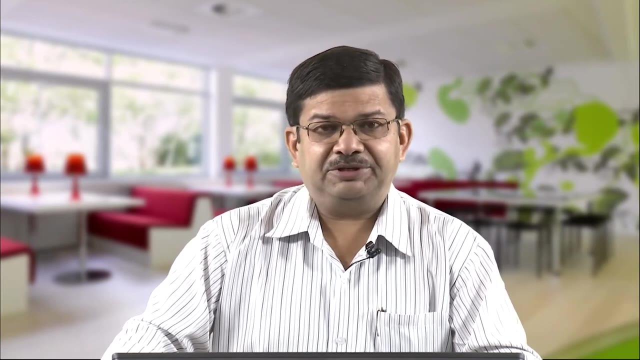 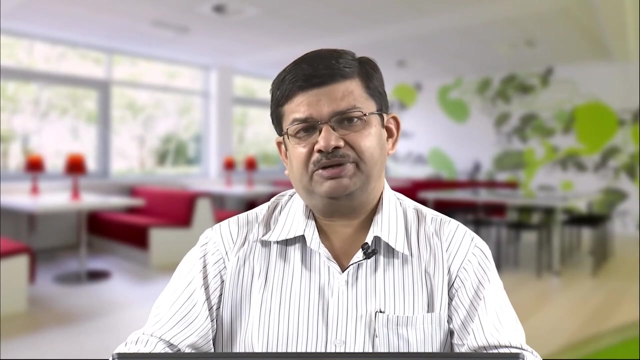 careful study of the influencing environment, the system per se that we are looking to design, and what are the operating conditions of the system, what are the parameters, operating parameters of the system, and so on. So it is a very complex system. There are lots of influencing parameters and there are cause and effect relationships between. 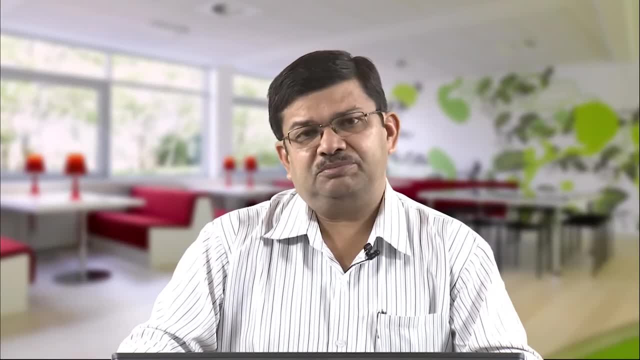 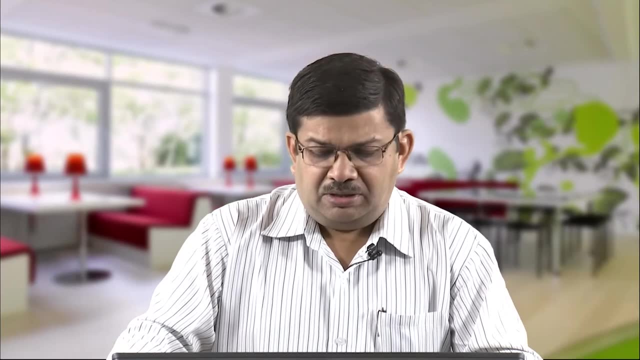 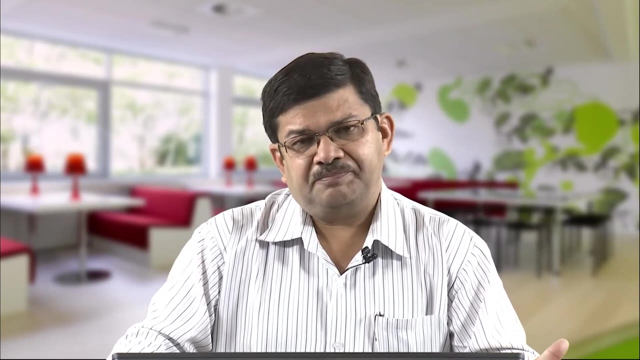 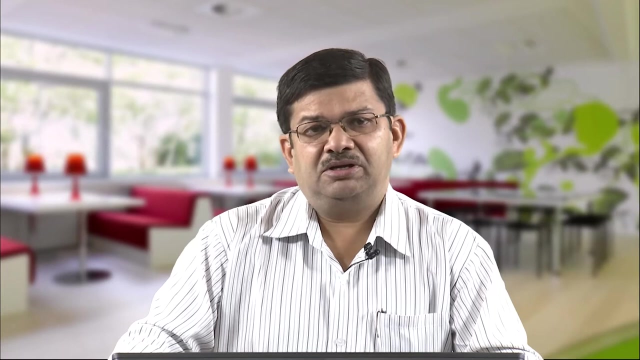 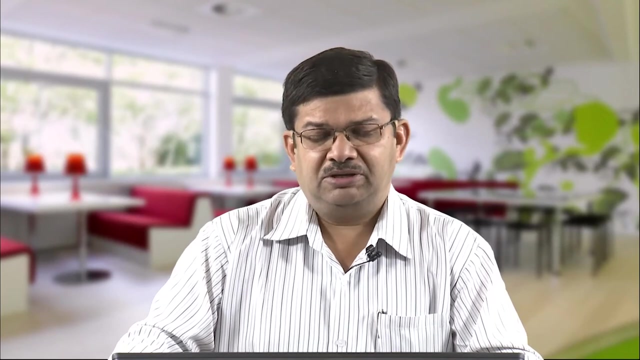 the system output and the input that it takes from the environment, conditions or the operating conditions. So obviously, this complex physical model, it is a very large system and it needs to be transformed into a mathematical model. So this is the basic model, with suitable assumptions within a suitable framework. assumed framework. 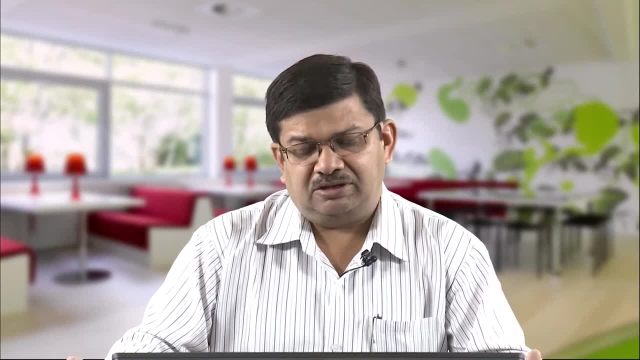 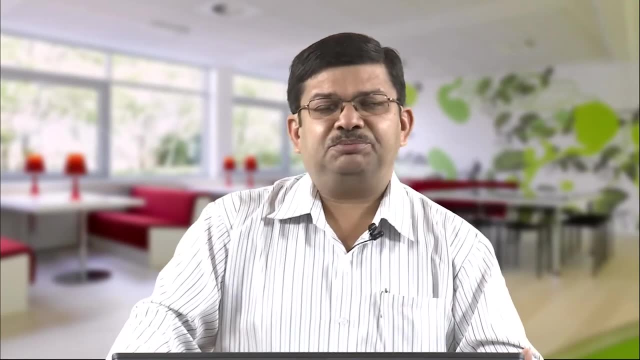 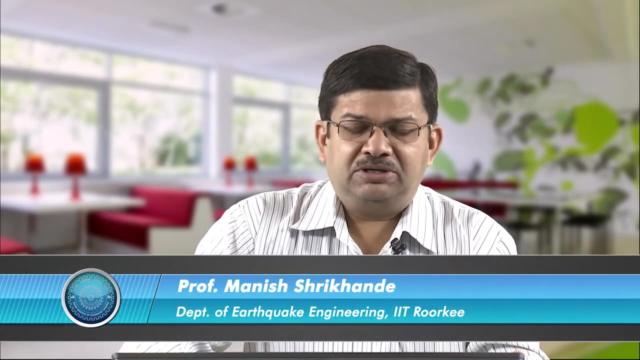 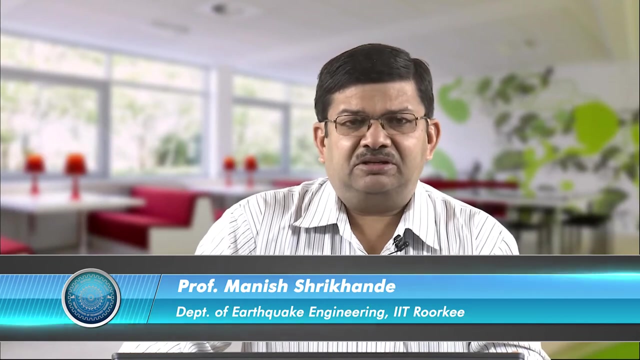 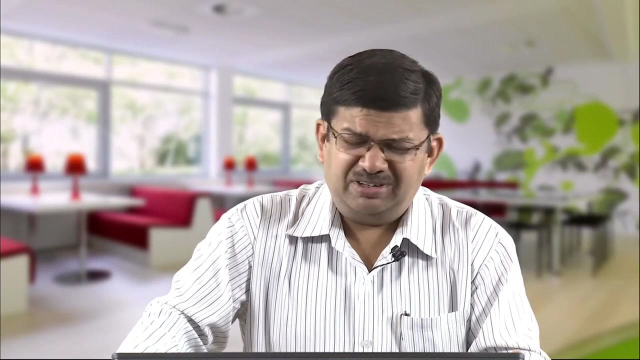 of certain idealizations such that we retain what are the significant influencing parameters and what are the significant variables of the problem. that will adequately capture the basic essence of the problem. We never try to model everything in Absolute detail. I mean very common maxim that is often quoted and often attributed. 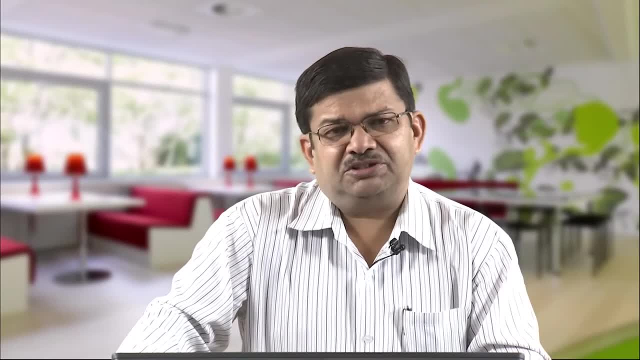 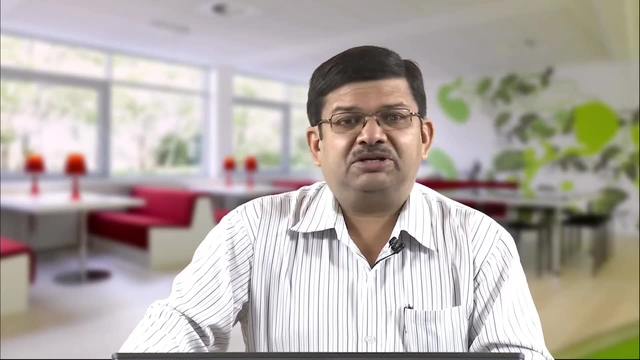 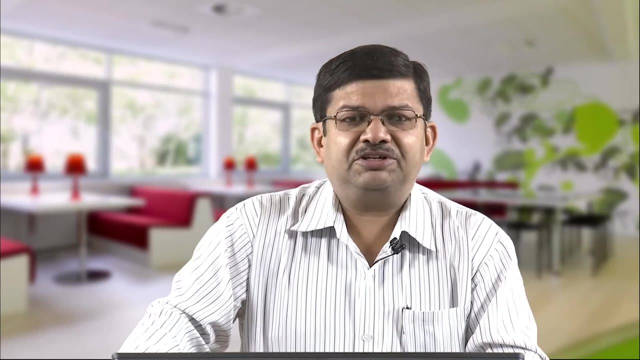 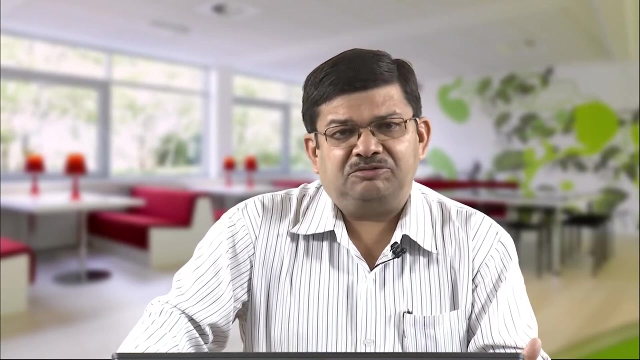 to Einstein, is not very sure about the authenticity. A model should be as simple as possible, but no simpler. So we need to have all the influencing parameters, all the significant parameters that have considerable influence on the operating conditions and the output of the system, and 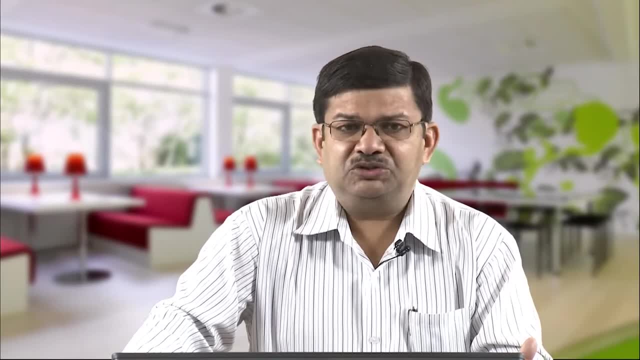 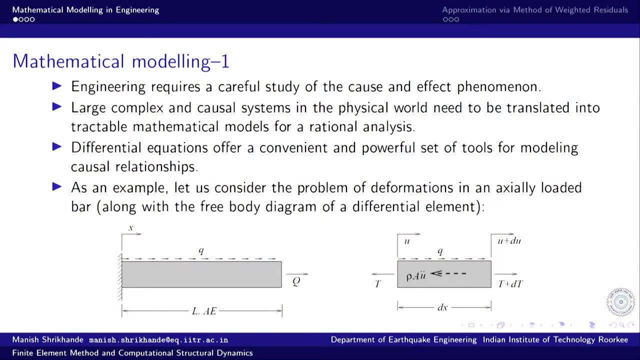 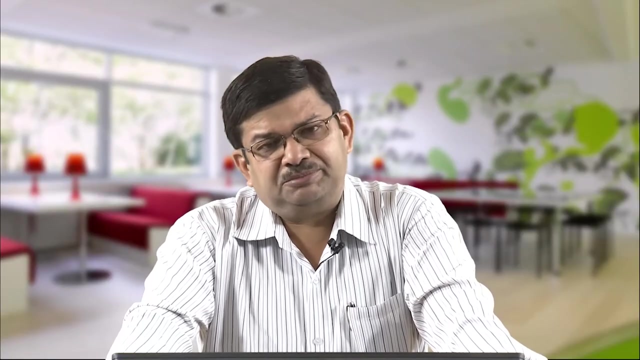 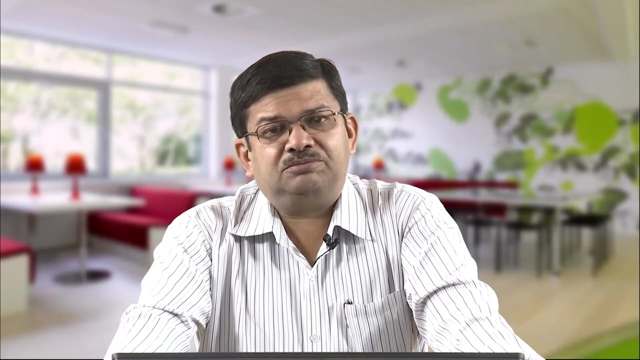 construct as simple model as possible using all these influencing parameters. So the basic idea, the first step towards engineering analysis, is to convert a large, complex and causal system in the physical world to a set of tractable mathematical models for a rational analysis. Mathematical models are amenable to our basic tools of mathematics and, of course, amenable 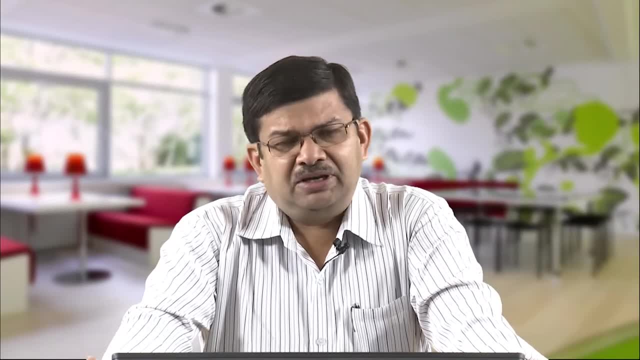 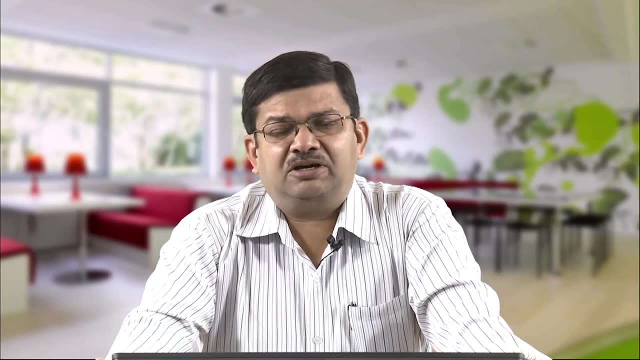 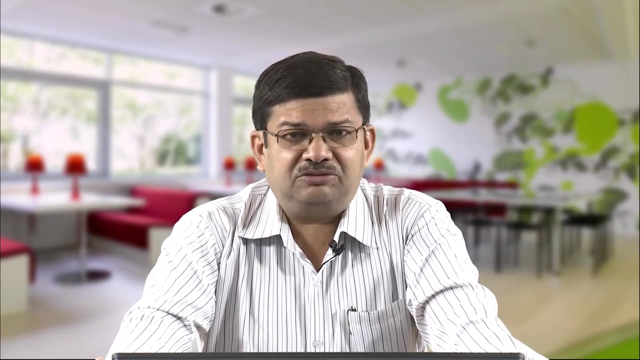 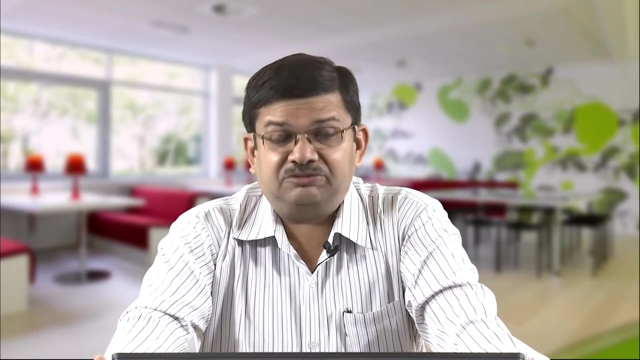 to treatment via digital computers and it allows that mathematical model allows itself to be studied under the influence of various operating conditions, which may not be possible to do in case of physical world. I mean, a physical experiment is very difficult to perform, it is time taking, it is very 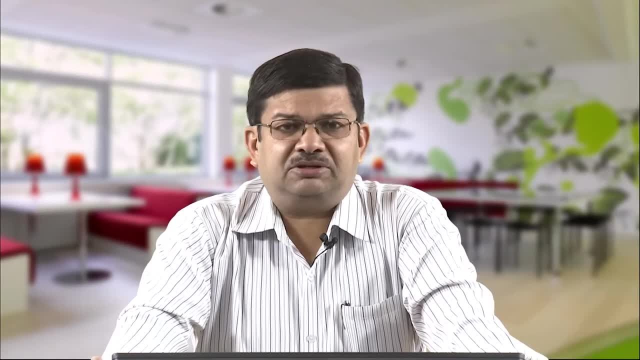 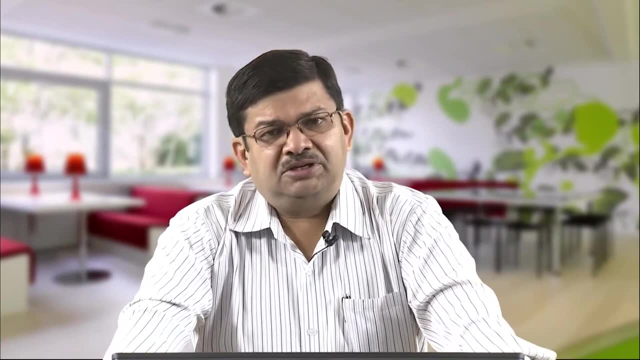 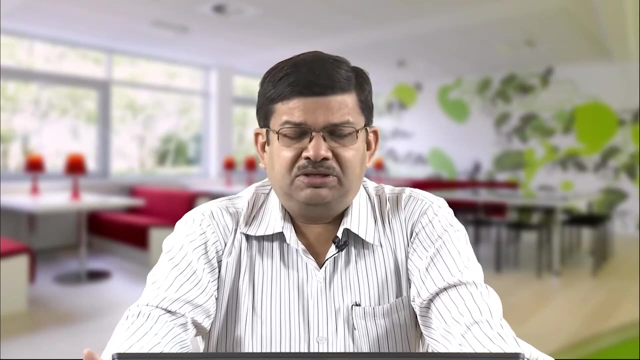 expensive and sometimes it may not be possible, A large scale system, for example a complete aircraft. it is impossible to test a complete aircraft prototype in a laboratory, But if we develop a mathematical model then it is possible to see what are the influencing. 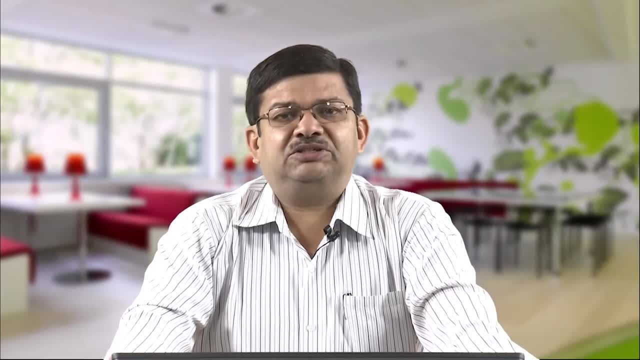 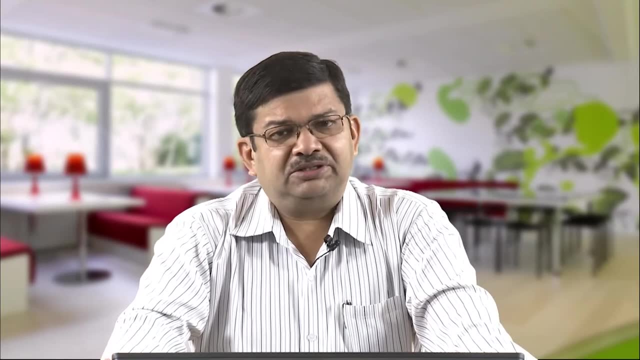 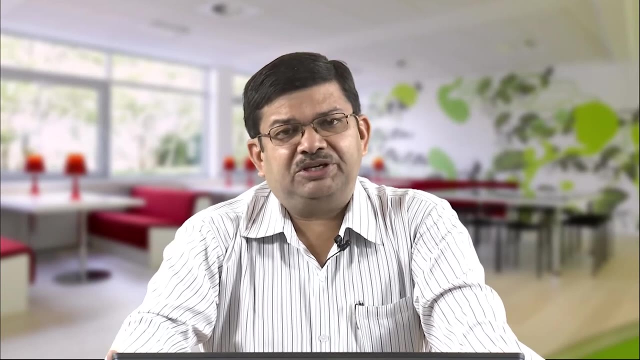 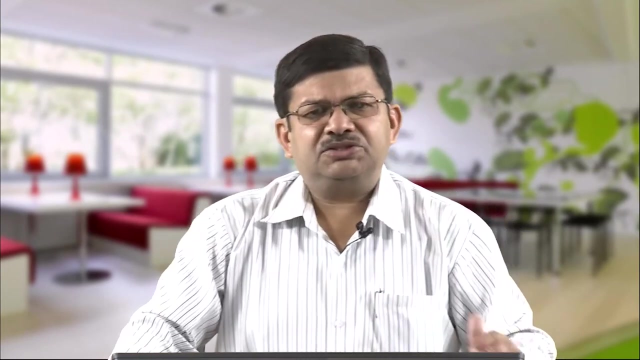 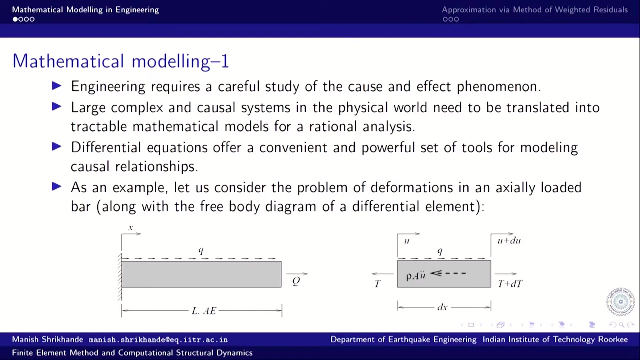 parameters how the complete system interacts with the environment that it has to operate on and appropriately take- I mean learn, draw inferences, learn from the results how the system behaves and then take appropriate call on modification of design if required. So the essential ingredient of this development of mathematical model is a differential equation. 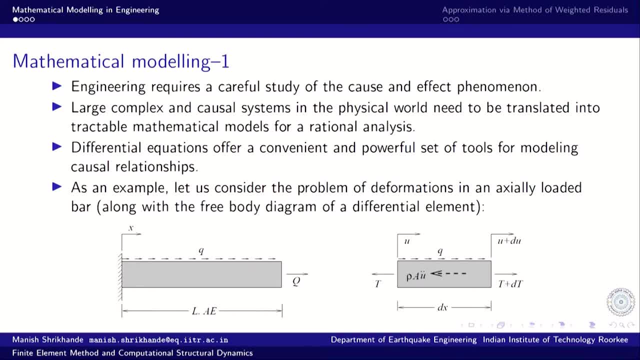 Differential equations. they offer a convenient and powerful set of tools for modeling causal relationship, If something is known to be dependent on certain things, certain variables. So we have a system of dependent variable and independent variable and we study and establish So the rate of changes, and that effectively gives us the basic differential equation of 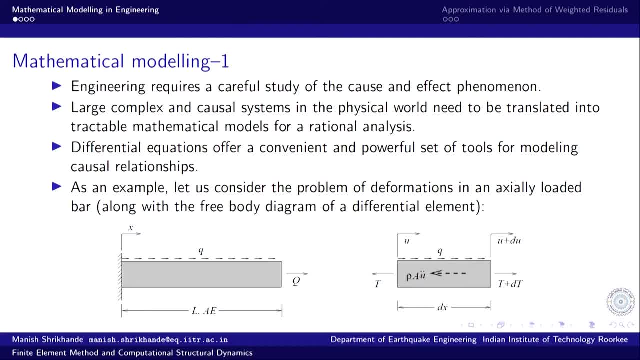 the phenomena. As an example, let us look at the very simple- I mean simplest possible problem in mechanics, that is, the axial deformations of a bar, as we see in this figure. So this can represent several things. it is a simple bar element or truss element, or 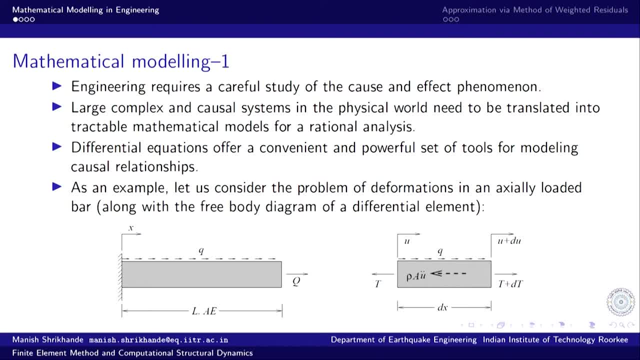 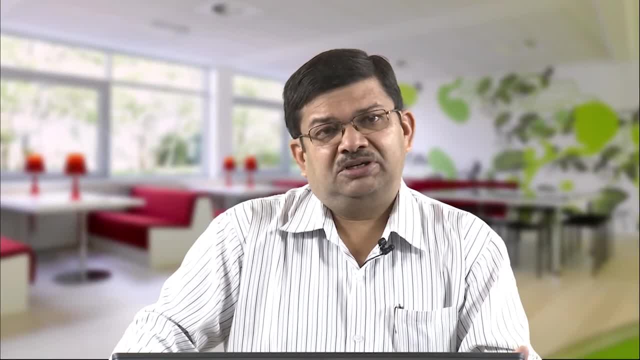 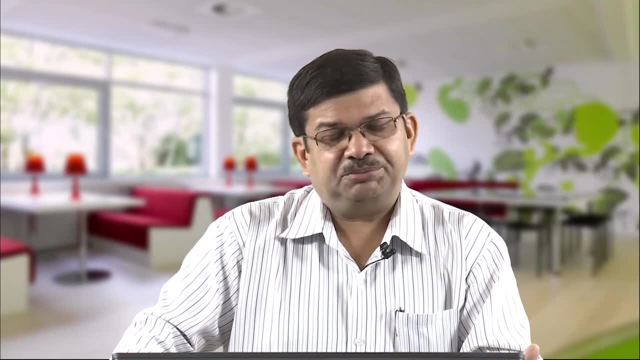 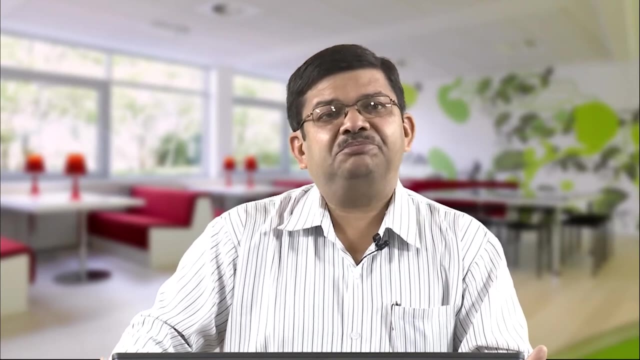 member of the truss That you see. for example, you might have travelled through several rail bridges. So each element, each member of that bridge, is modeled as a truss element and that is a bar under axial deformation. Another situation is particularly this particular example that refers to end bearing piles. 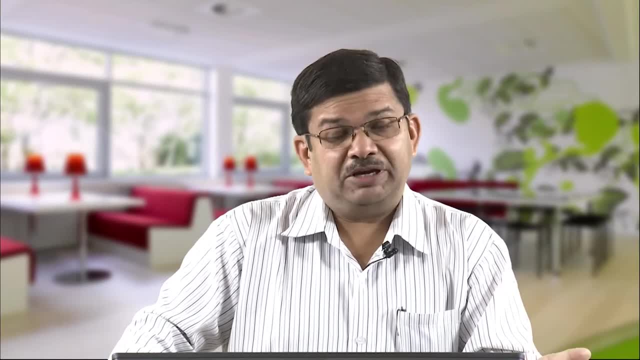 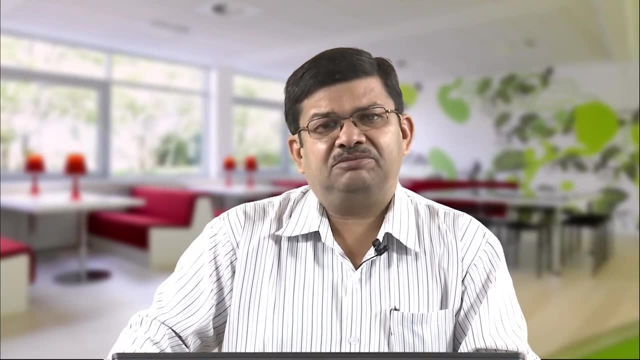 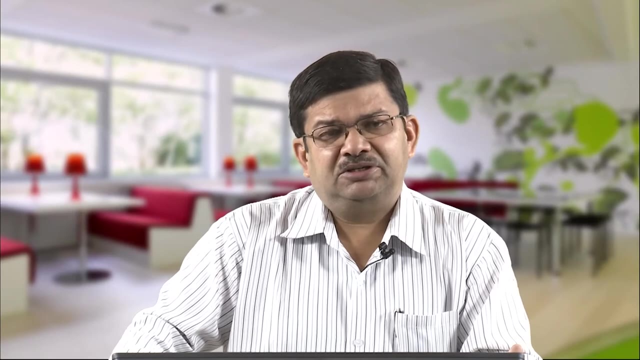 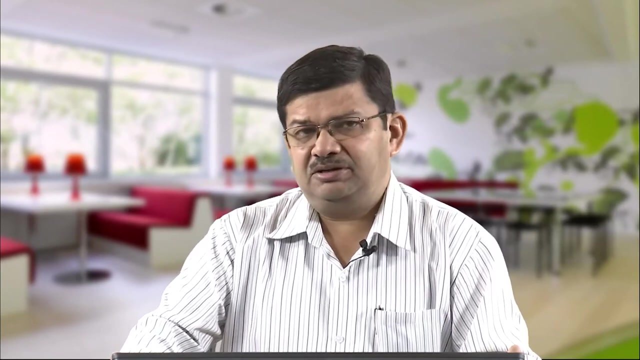 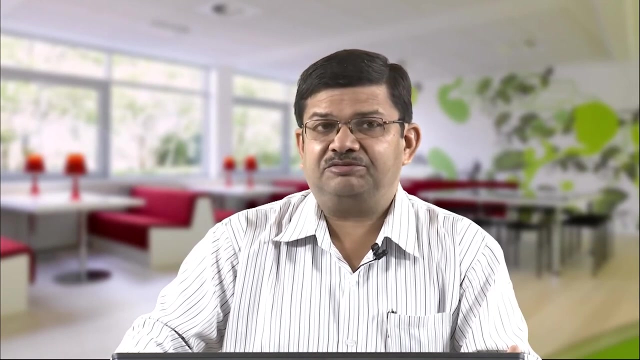 So the problem of driving a pile through the pile foundation. 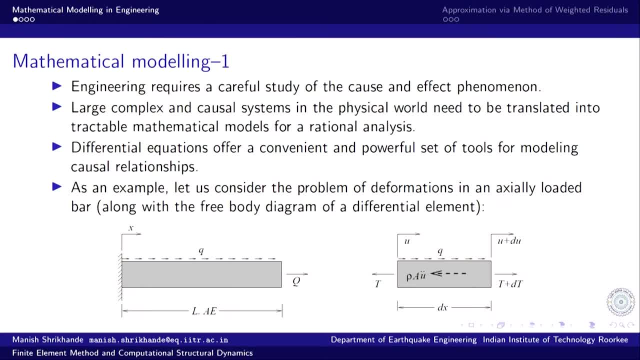 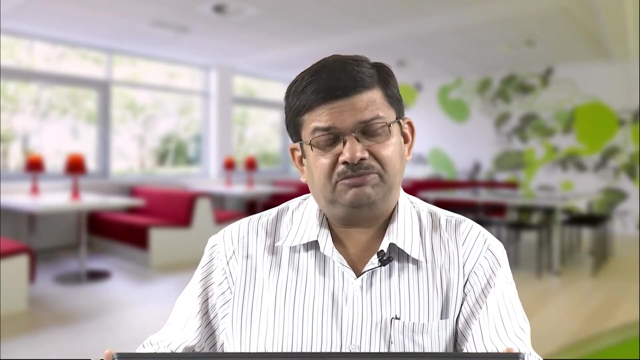 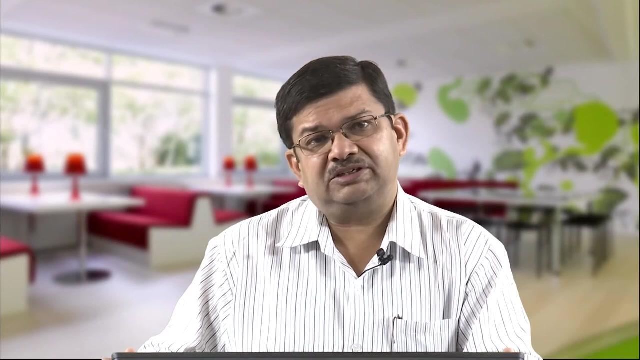 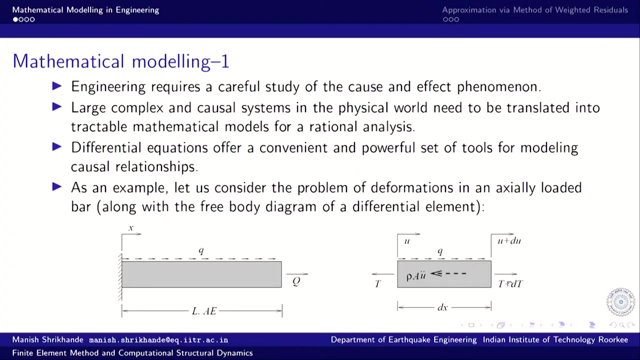 that occurs between the surrounding soil and the pile surface. So because of this skin friction, there will be a difference in the axial thrust and, of course, if the deformations are time variant, then we need to look at these basic mechanics. 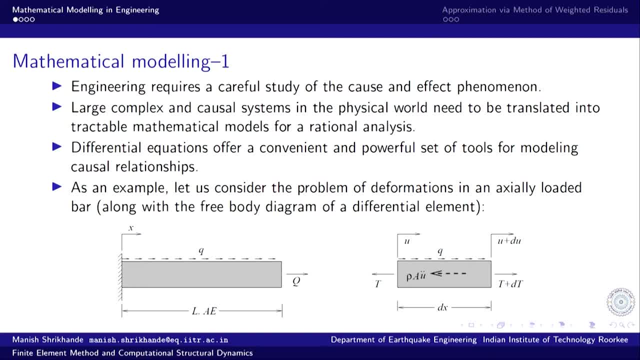 Newtonian mechanics, second law of Newton, and Newton's laws of motion, the law of momentum, all forces in the body. they are equal to rate of change of momentum of the body. So this is rho A? u double dot. that is essentially rho rate of change of momentum. and in this 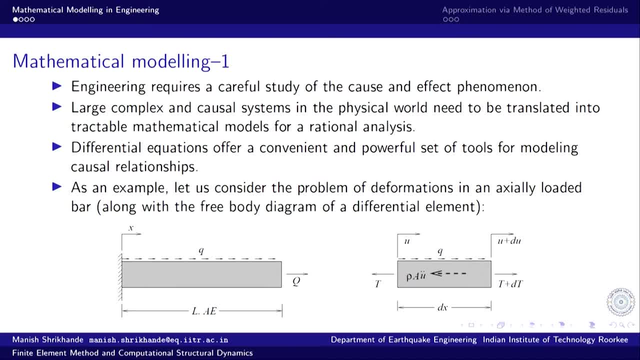 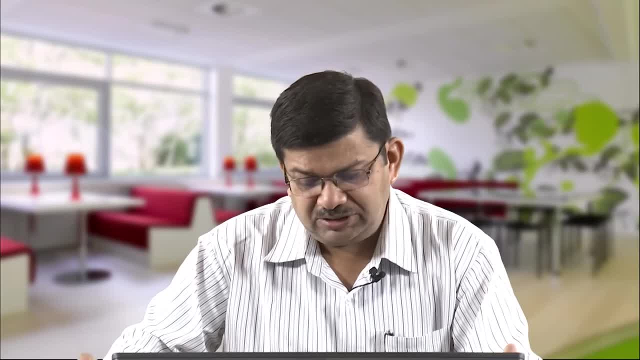 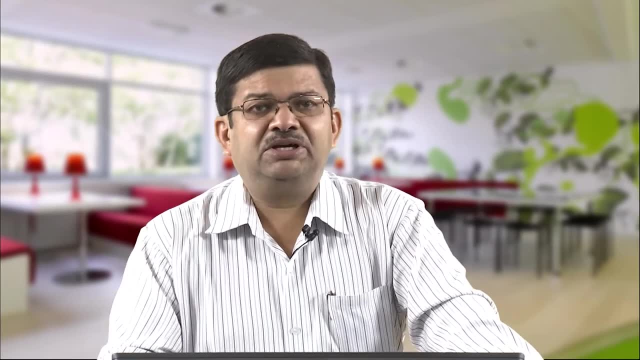 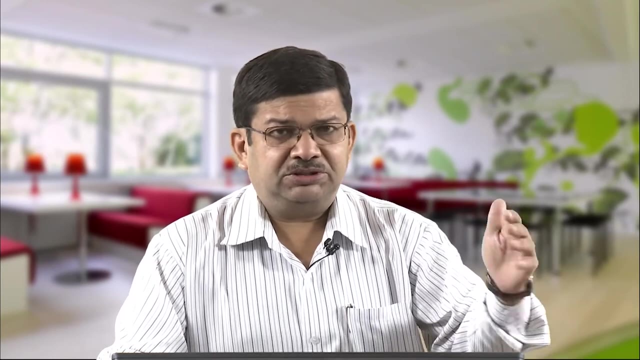 case particularly, it is shown as a dotted line as a fictitious inertia force. So inertia, force, the force, the nomenclature. it is very common in the parlance, structural dynamics parlance, to refer to inertia term as a force term. Because in the equilibrium, Newton's second law of motion, left hand side, you have the 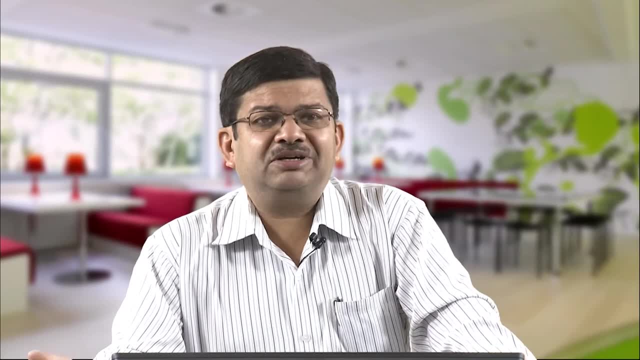 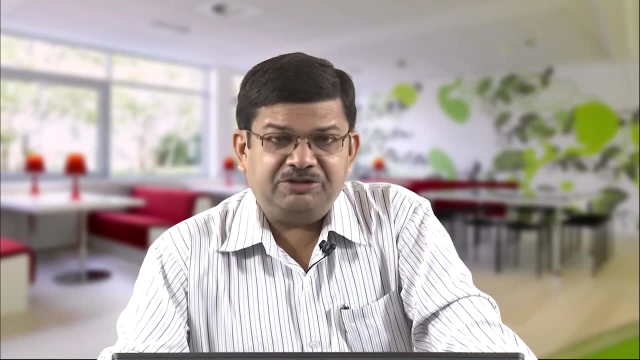 force terms and on the right hand side you have rate of change of momentum. So it is dimensionally consistent. So it is equal to the Applied of total applied forces. but still it is not a force, it is a separate law. it. 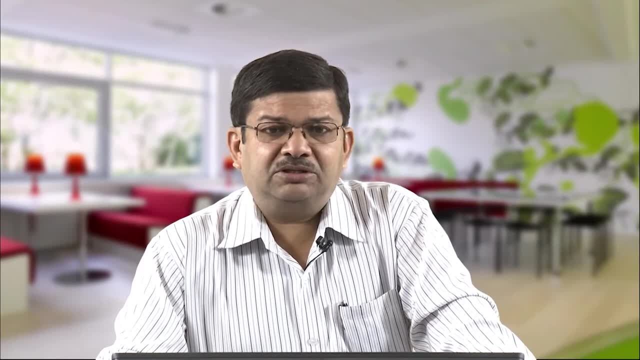 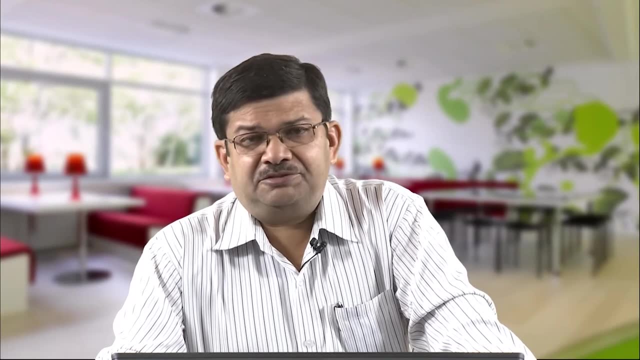 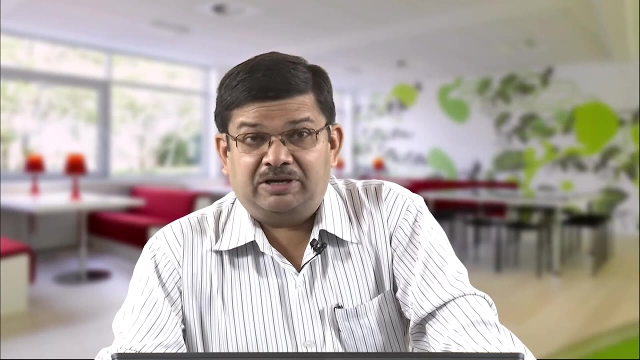 is a law of momentum, So all applied forces on the body they are equal to the rate of change of momentum. Now why is it not a force? because this particular rate of change of momentum that we have, it happens to have the units of force, and that is why it is left hand side- is equal. 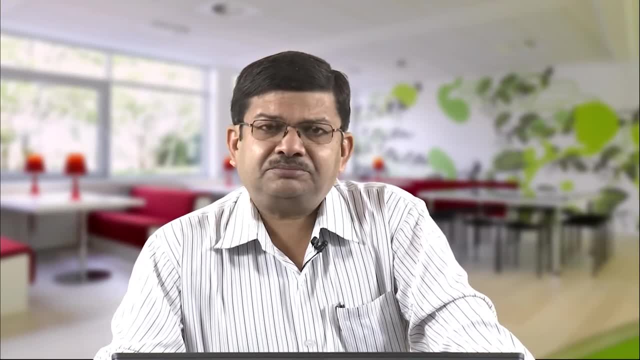 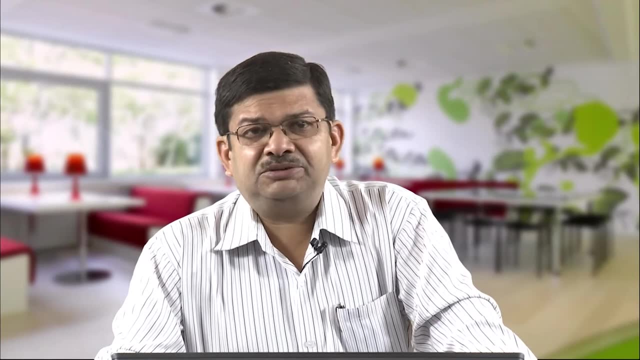 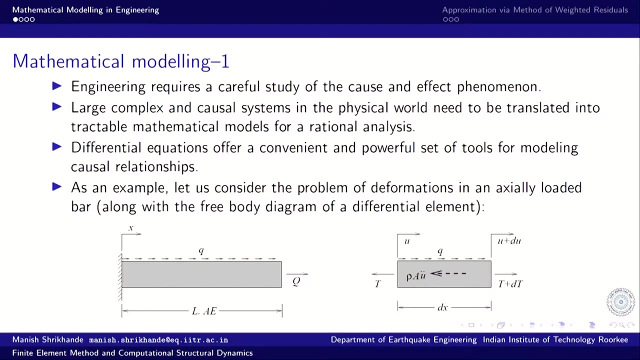 To right hand side in the Newton's second law, but it violates Newton's third law. there is no reaction to this force. if this was a force, if this rho a? u double dot, if that was a force or action, Then by Newton's third law it has to have a reaction. and there is no reaction for this. 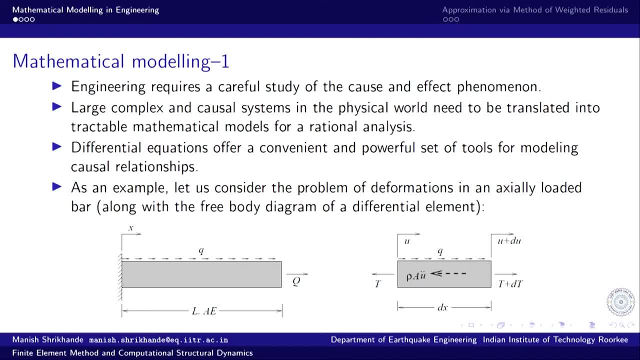 and that is why it is often Now, if we refer to- I mean if we look at- the force equilibrium statement, then it is convenient to treat it as a force, but it is always made a distinction. It is drawn as a dotted line just to indicate that it is a fictitious force and we are talking. 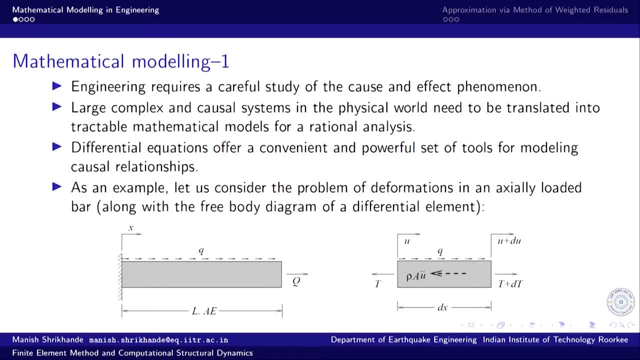 about an equivalent representation of force, equilibrium, instantaneous equilibrium by D'Alembert's principle, and we can treat that as a force and just treat it as a static equilibrium at holding at each instant of time, So using this rate of change of momentum as a equilibrium. 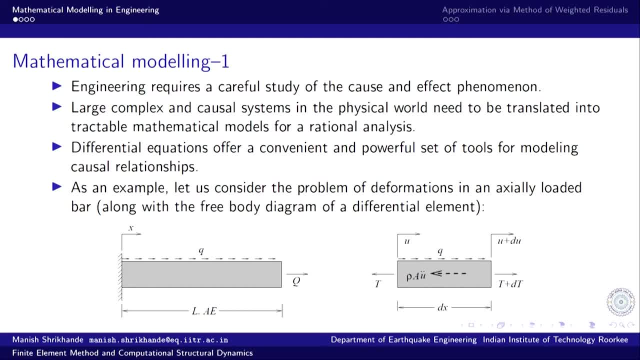 force, inertia force, fictitious inertia force. and that works because in the case, in this particular case, rho A u double dot. it is a mass is time variant for most of the system, except for aeronautical systems where significant amount of mass comes from the fuel and fuel. 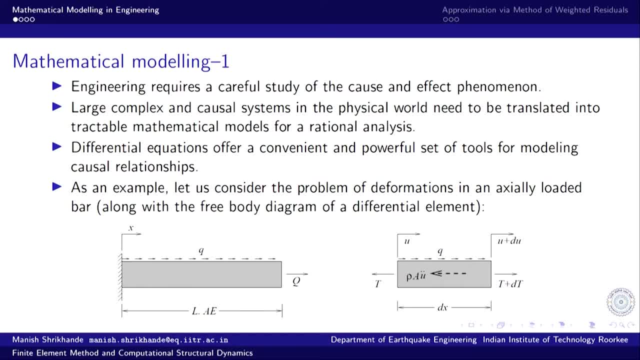 is burning at a rapid rate to give the thrust that it needs, and therefore rate of change of momentum is actually dependent on the rate of change of mass as well. So for aeronautical systems situation is little more complex than what is presented here. there will be one more term that is dependent on the rate of change of mass, But 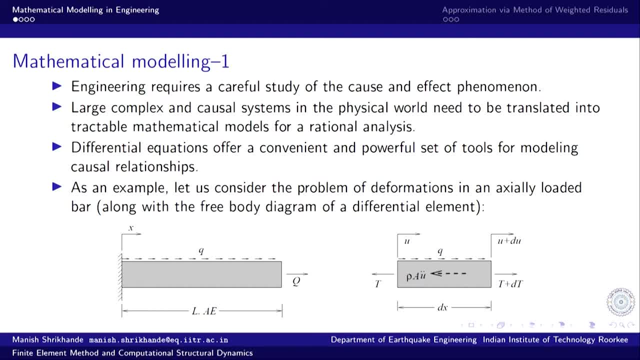 let us remain anchored to the ground, and for most of the problems that we deal with in civil engineering and mechanical engineering systems, the mass is time invariant and the second law of motion, the rate of change of momentum, essentially refers to mass times acceleration. So if we establish this equilibrium, consider this equilibrium and collect the terms together. 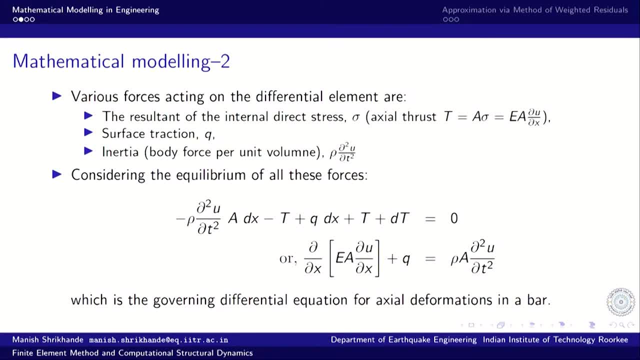 then we can develop the equilibrium equation. So, as you can see, the various forces act on this differential element, as I mentioned, resultant of the internal direct stress sigma. so that is axial thrust area times the direct stress, and that is, of course, equal to by making 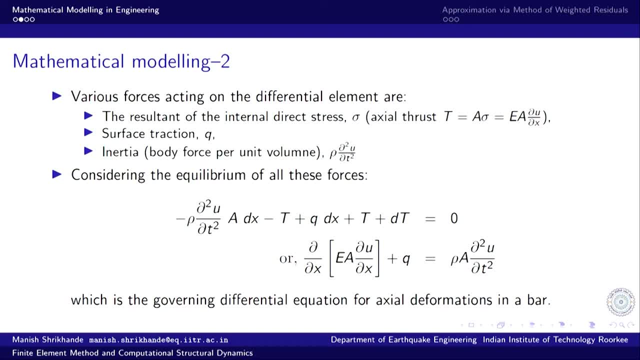 use of Young's, modulus and Hooke's law. So axial thrust is equal to Ea times, direct strain del u by del x. Now this axial thrust element can be calculated by adding the corresponding 2 p and b to Ea times delta square root of delta u. So this is the axial thrust element and we take the definite energy of that radial force made of Ea and delta, square root of delta, square by Ea, as equal to B byGA, then you can be anderenly, but you can also integrate all these terms by that. so an initial strength will be Ea by 2 into this Ay, by gamma, by 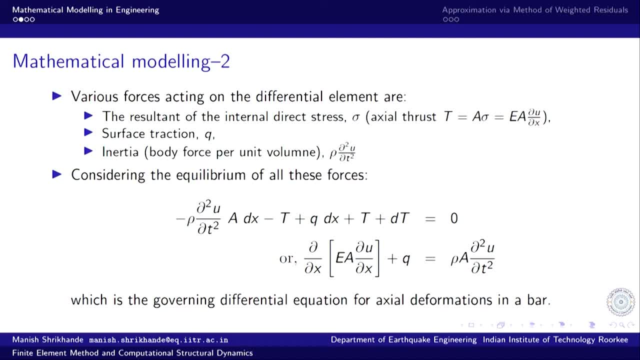 2, and by gamma, by omega, by of delta square root of delta. square root of delta square is equal to Ea by 2. the only definite it is the constant force. Then there is a surface traction distributed on the circumference periphery of the body. 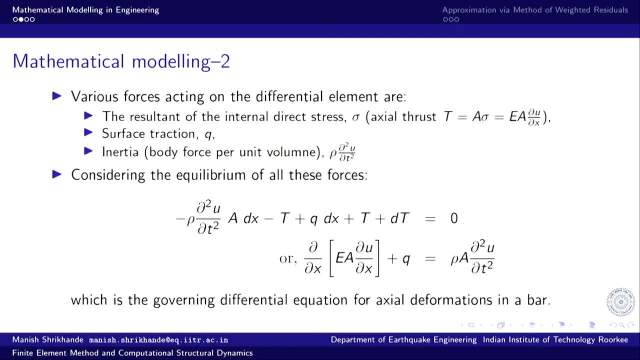 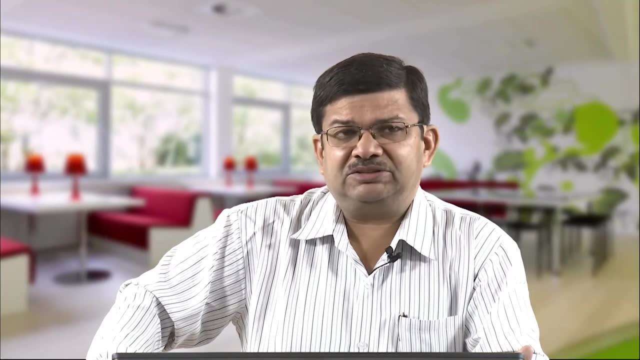 and inertia. so the body force per unit volume, and per unit volume the Ax, that is the volume of the differential element Adx. So per unit volume it would be rho times del 2u by del t square, that is u double dot. so acceleration term. 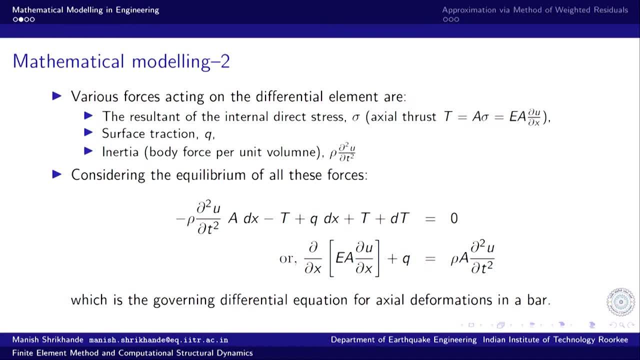 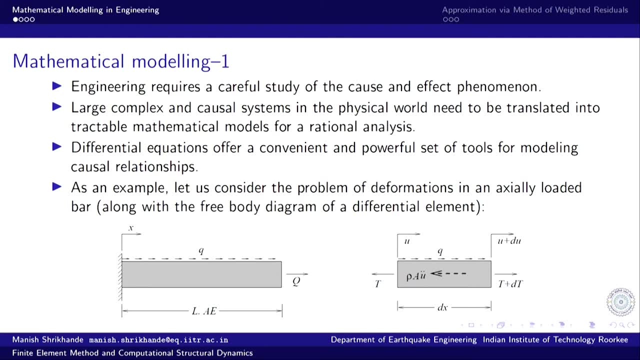 So, if we consider all the equilibrium of all these forces, so considering the D'Alembert's principle, the inertia force- fictitious inertia force- acts in the direction opposite to the direction of motion, so it has to act in the opposite direction. 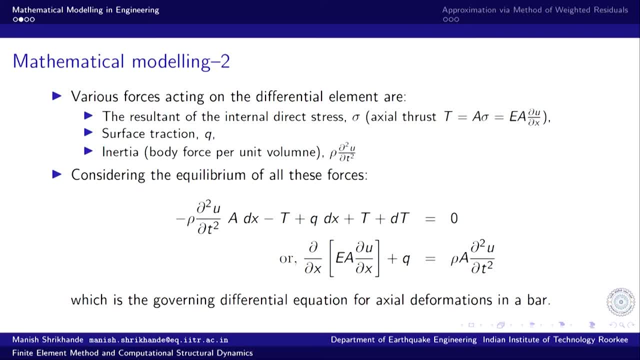 So, considering the equilibrium of forces, instantaneous equilibrium of forces, and then dividing through by the length differential element dx, we arrive at this governing differential equation. So del over del x, of EA, del u by del x plus q is equal to rho a del 2u by del t square. 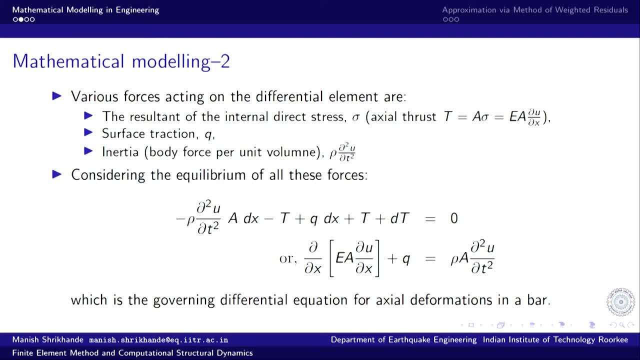 So that is the governing differential equation of the axial deformations in the bar And, as you can see, this is a second order differential equation. The highest order of derivative that you see is 2, with both respect to spatial derivatives as well as. 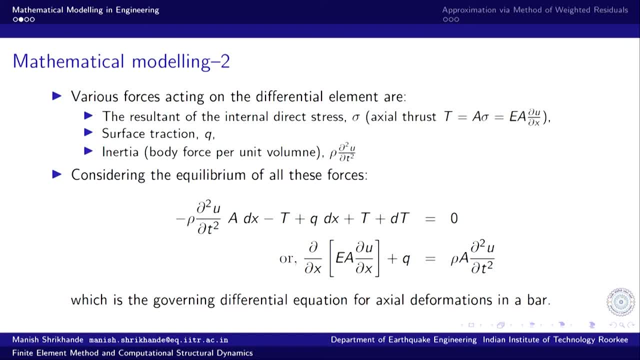 with respect to time derivatives. Now, there are two independent variables here: spatial variable x and time variable t. So there are. that is a complication that we would like to avoid getting into at the moment. We will deal with time dimension subsequently. but to keep matters simple, let us consider: 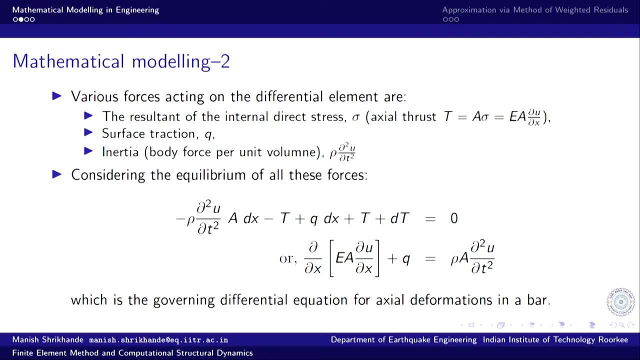 the situation in which the deformations vary slowly with respect to time. So if the deformations do not change very rapidly with respect to time, then the acceleration term is going to be negligible. So del 2 u by del t square, it is going to be a very small quantity and therefore we 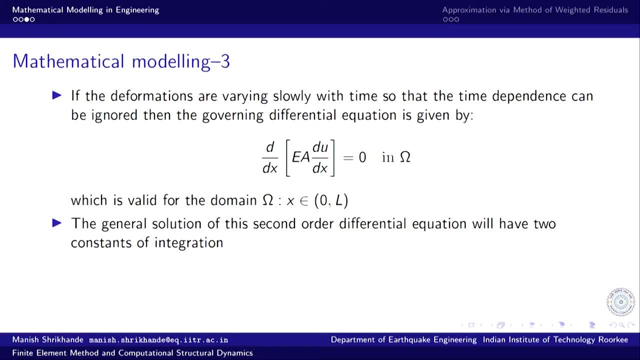 can ignore that term- and we can- we are left with an ordinary differential equation. So the governing differential equation now reduces to an ordinary differential equation because there is only one independent variable now. So d over dx of ea, du by dx is equal to 0 in omega. 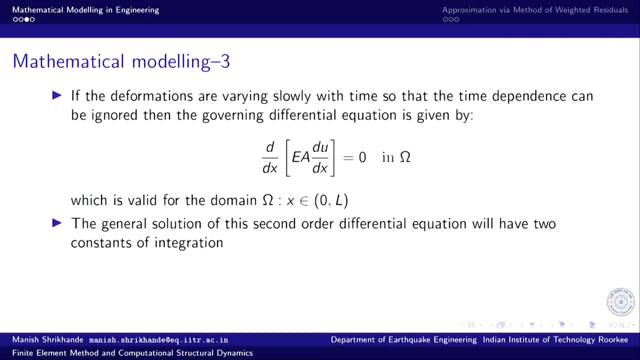 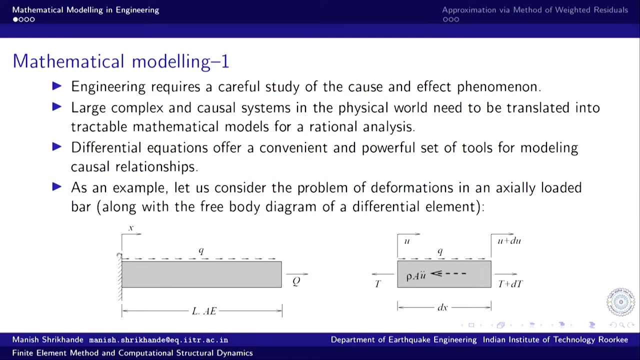 Now that is an interesting addition to the whole thing. Starting from x is equal to 0 to x is equal to L. So that is the extent of the problem, range of the problem or domain of the problem. So that is the domain over which differential equation, this particular differential equation, 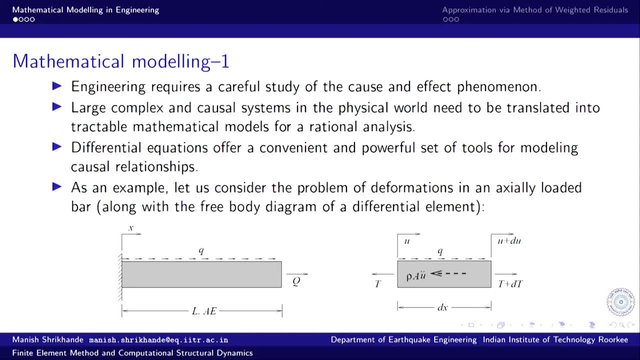 holds. So every differential equation that we develop has to have a particular domain over which it is what is the range of applicability of that differential equation? and that has to be specified with along with the differential equation. A differential equation has no meaning unless we specify what is the domain of its application. 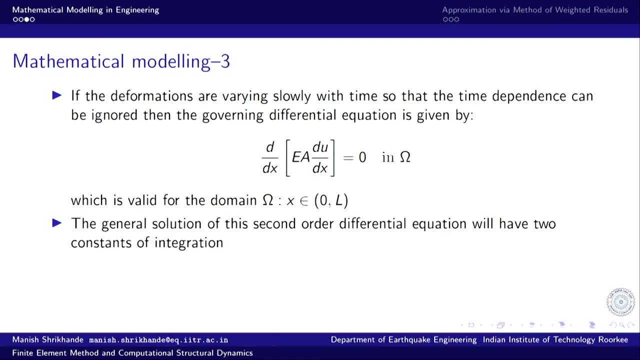 Now this is, as I said, it is a second order differential equation and obviously it will have two constants of integration. So that is general solution. The general solution of this second order differential equation will have two constants of integration and obviously we will need two boundary conditions, two additional conditions. 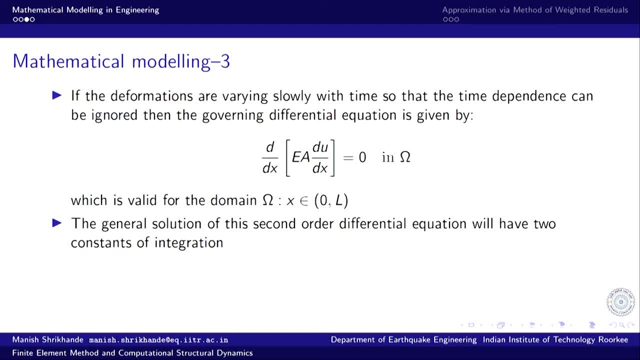 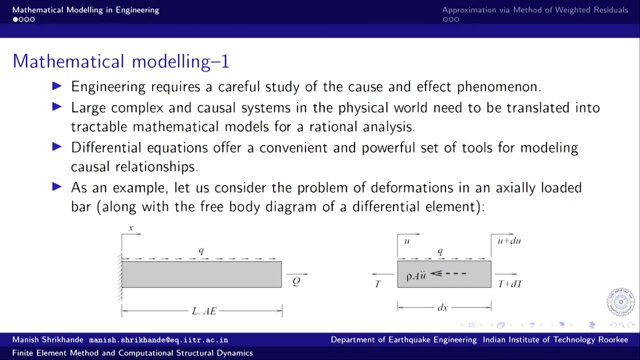 to determine specific solution. What is the specific solution to the problem? What do I mean by specific solution, For example? let me go back to the equation- A solution will be different If I removed this. I have this fixed boundary here. 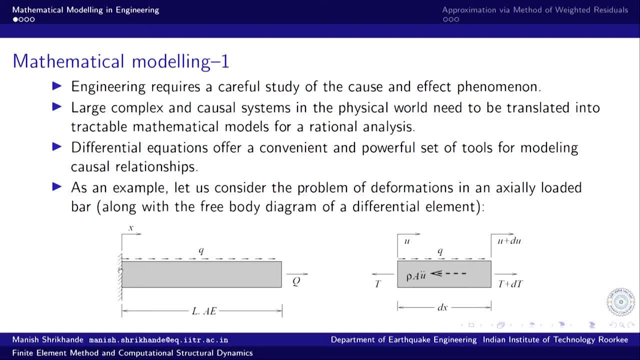 If this fixed boundary was removed and made a free boundary. that is a different problem than what is presented here. Secondly, if I remove this force here and then apply a, if I remove a force here, leave it as it is, that is a different problem. 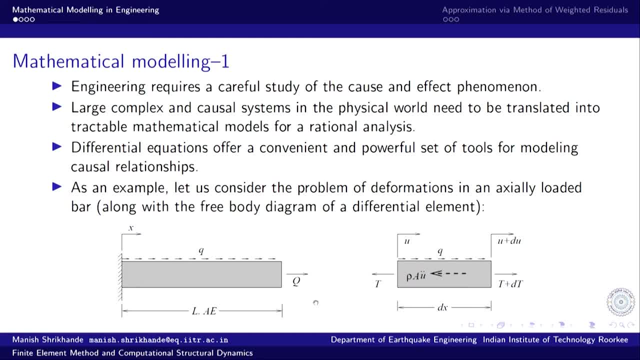 If I apply a constraint here, Put some value, either restrain it from displacement or make it some other value, non-zero, so prescribe some deformation. at that point that becomes another problem. So while general solution as a differential equation I can have a general solution. 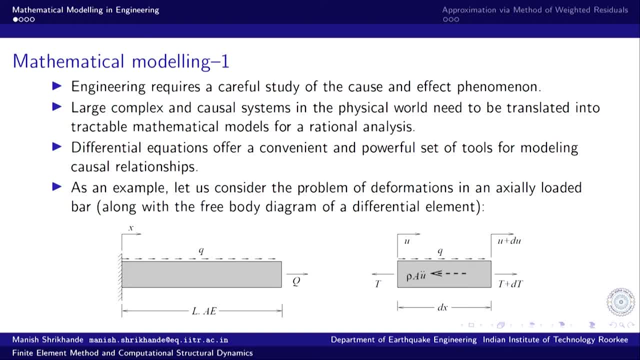 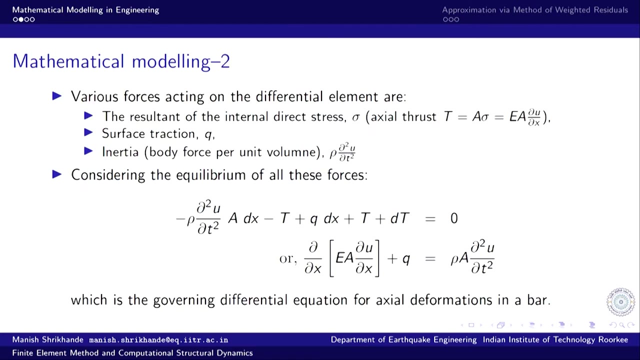 But for each of the specific problems that can arise because of the peculiarities of the situation There has to be, There will be specific solution for each of these peculiarities. Now, those specific solutions are captured by appropriate evaluation of the unknown coefficients of, or unknown constants of, integration. 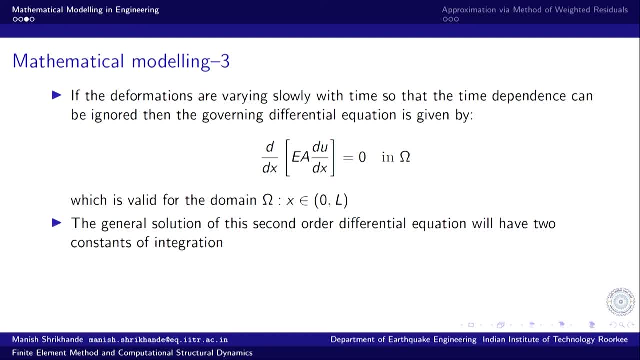 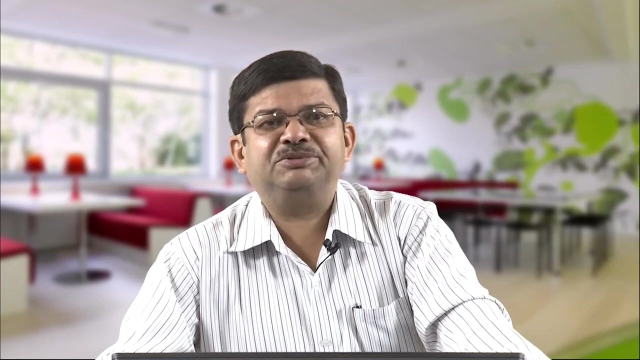 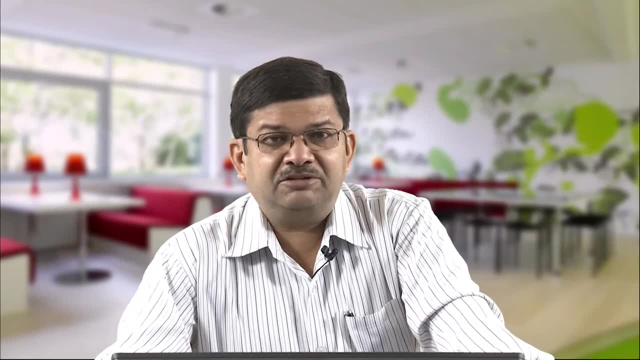 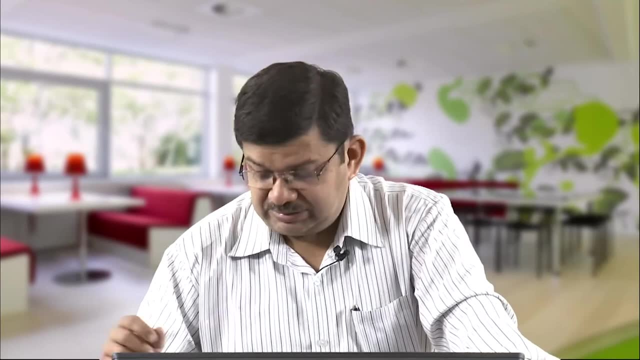 to solve. So in our bar problem that we have, the boundary conditions that we have specified are: u at x is equal to 0, that is, at x is equal to the origin of the problem. so this is x axis is measured from here. 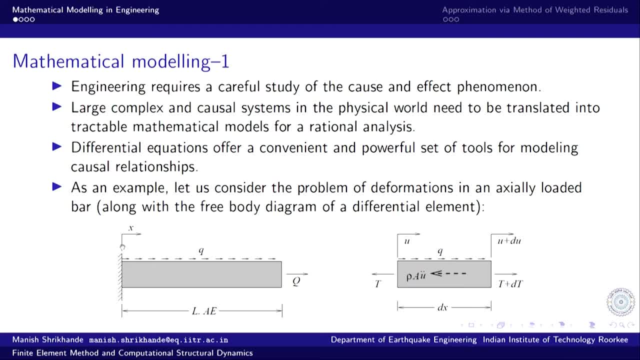 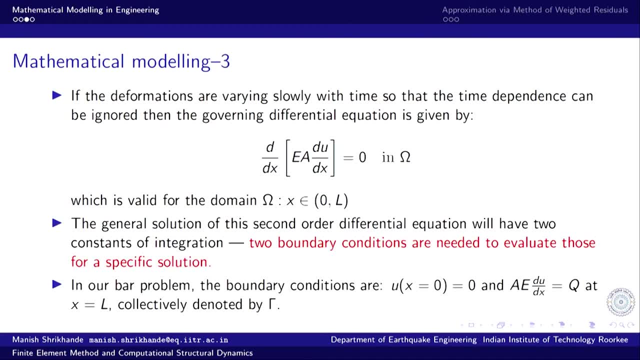 So at this particular point the deformation is held 0, is constrained to be 0.. So that is the one boundary condition. So in our bar problem the boundary conditions are: u at x is equal to 0, u is the basic unknown. 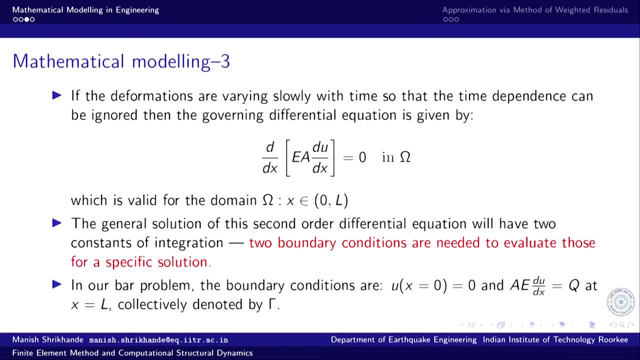 of the problem: the deformation, axial deformation of the bar. So axial deformation of the bar at x is equal to 0, is 0 and the axial thrust, So A e d x is equal to 0.. So A e d x is equal to 0.. 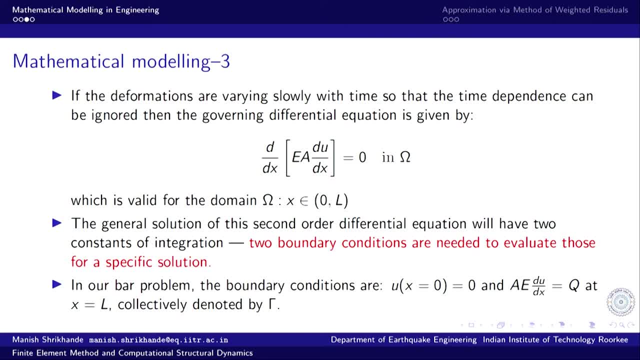 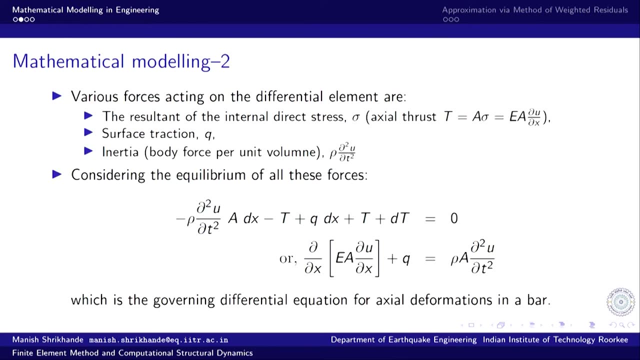 A, e, d x is equal to 0 and d? u by d x. that is the axial thrust. So the axial thrust at the free end, at x equal to L, is should be equal to Q, just to ensure equilibrium condition. otherwise the system will not be in equilibrium. 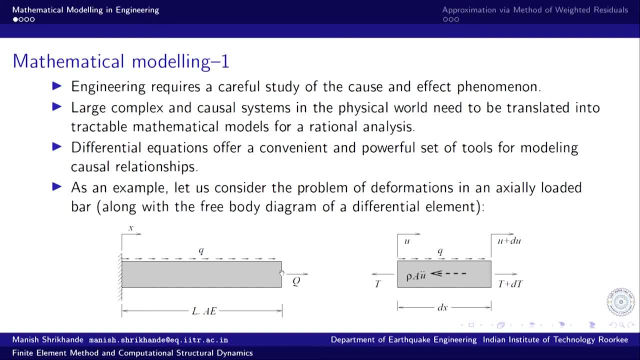 So at this particular points, whatever if the axial thrust here, that should be equal to Q. So that is the basic two boundary condition, itiek Yeah conditions, and that will define set of the basic set of two boundary conditions that. 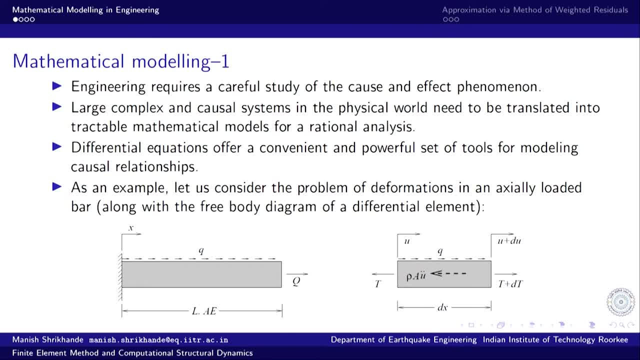 will define the specific solution to this problem. So a general solution to the second order differential equation will be defined, will be catered, will be made specific to this particular problem by evaluating the unknown coefficients of the problem, constants of integration which will suit the governing. 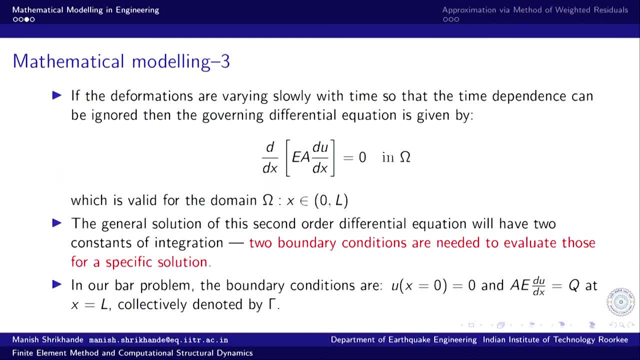 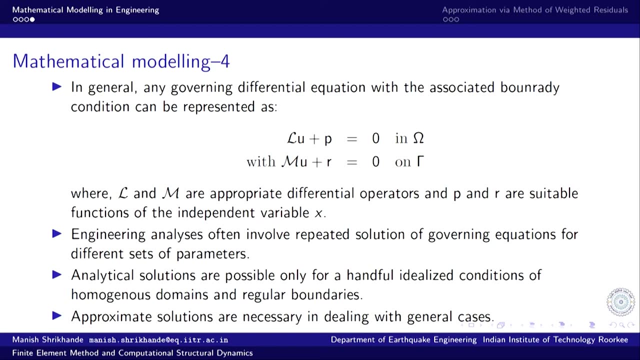 this particular two boundary conditions. So that is the in our boundary condition. these are the two boundary condition boundary problems and in general. so what we discussed was, with specific reference to a bar problem, second order, differential equation. Similarly we can. 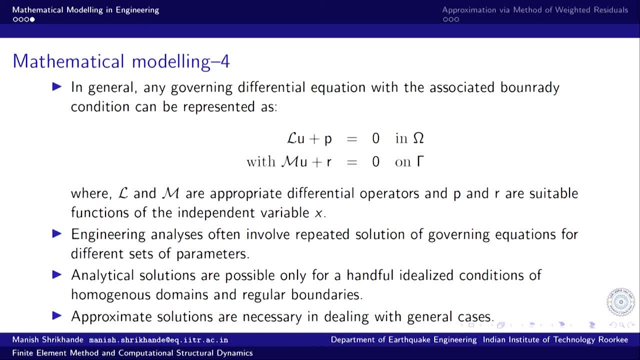 Develop similar formulation for any problem and in general it will be associated with some differential operator, let us say L, So this is differential operator. in this particular case our differential operator was second order differential operator. So d over dx multiplied by ea, again d over dx, and that is the differential operator that 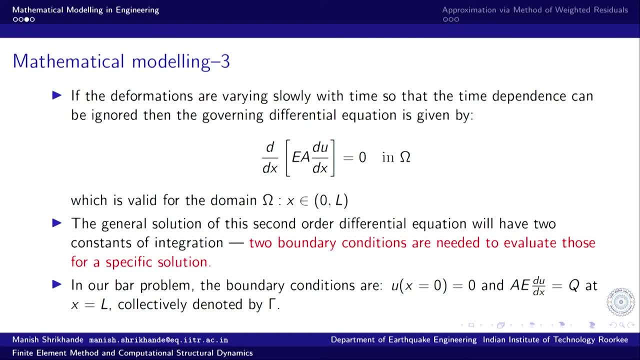 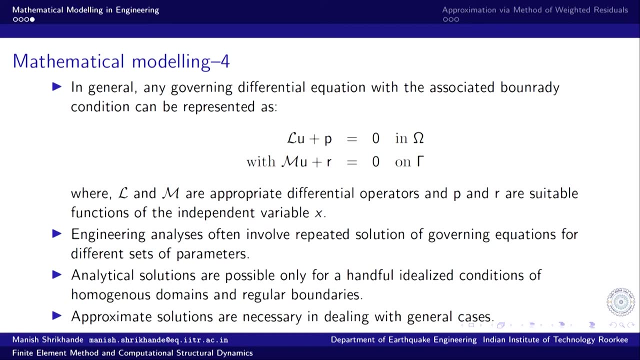 we have. So that is the, So this particular item, except a, u. this is all what we have as the differential operator, L in this case, and p can be anything. it is a function of independent variable. 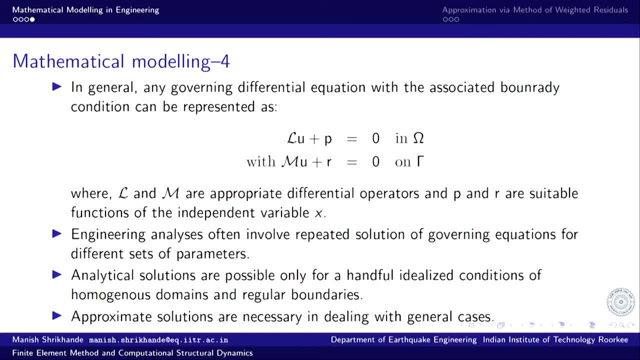 it is a suitable function. it can be a known function, it can be a constant or zero-third order function. So it is. that is how it is the problem. it is, the problem is defined, and that is equal to 0 in omega. So again omega. so the domain. 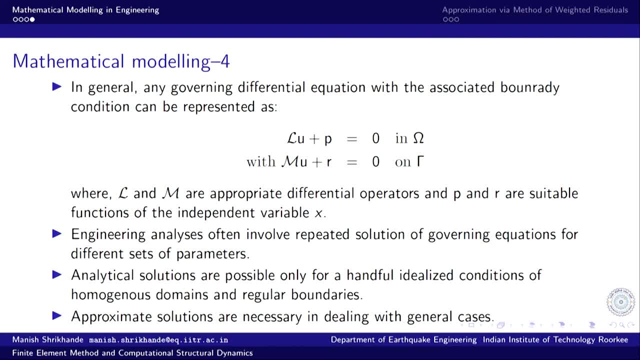 of application is defined. So this differential equation L? u plus b- L? u plus b is equal to 0 in omega- is the governing equation of any problem. It can come from anywhere. it can come from mechanics, it can come from fluid mechanics, structural mechanics, fluid mechanics. 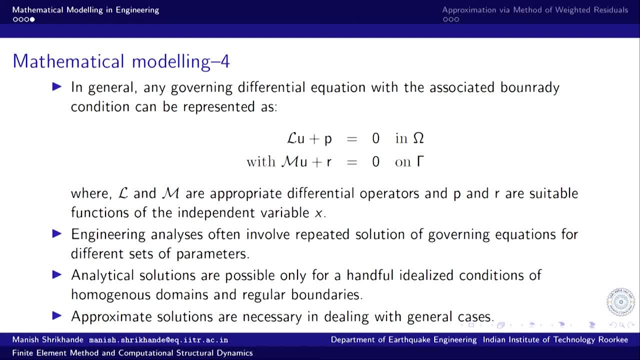 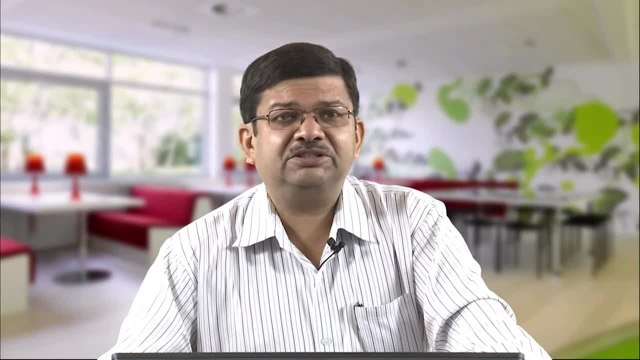 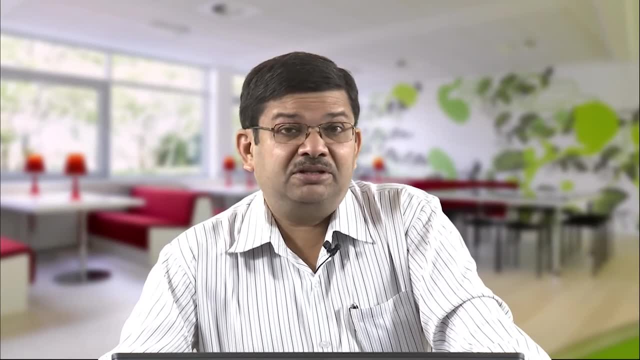 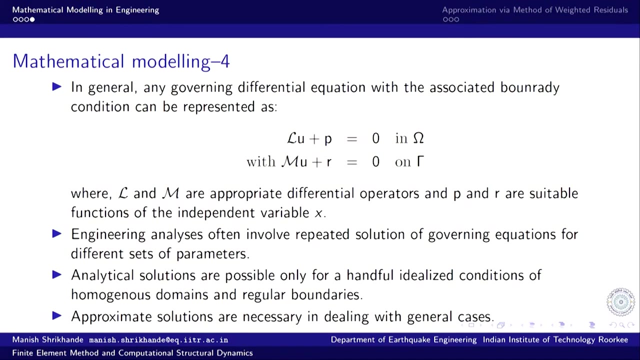 heat, conduction, electromagnetic, anything. so any differential equation And then obviously, as we discussed, general solution, differential equation will have a general solution, but the solution specific to the problem at hand will be defined by the boundary conditions. So associated boundary conditions are: m? u plus r is equal to 0. on 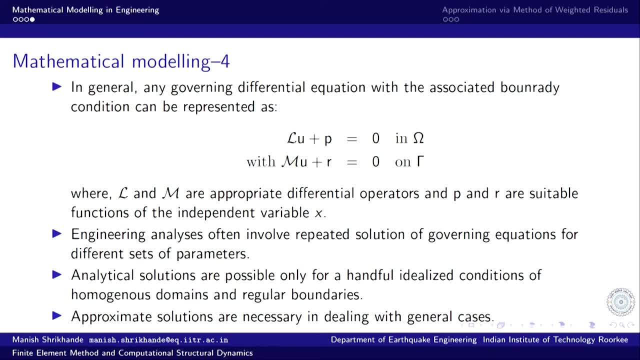 gamma. So we have this situation: domain is defined. It is defined by omega. Now the domain is enclosed by boundaries, So gamma is the boundary. So gamma denotes, I mean, it is a symbolic representation. So in case of bar problem, 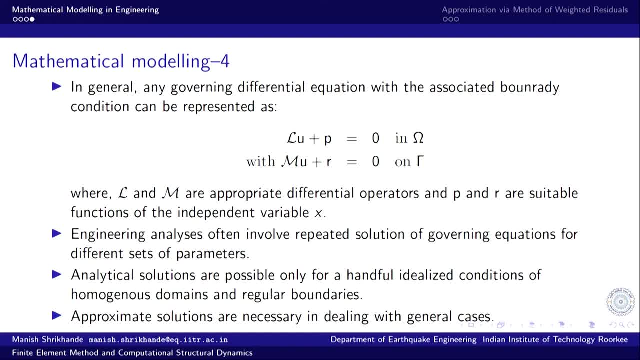 gamma constitutes two points, two end points: x is equal to 0 and x is equal to L. In between x is equal to 0 and L, we have the domain of the problem, So that is one dimensional problem. In case of two dimensions, we will have a curve. gamma will be a curve, So gamma. 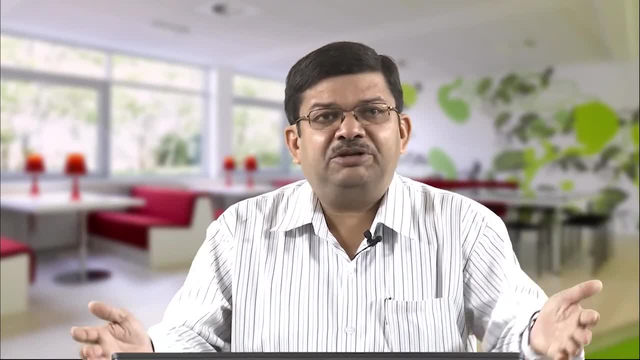 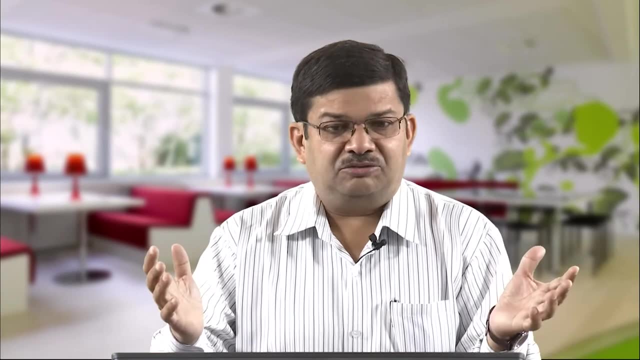 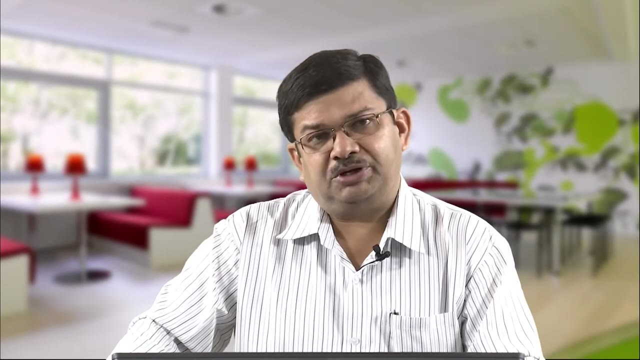 will be a curve which will enclose the area and the domain becomes the area. between these bounding curve In three dimensions we have a surface, boundary is a surface, and the volume enclosed by that surface becomes the domain of the problem. So the conceptually it translates: 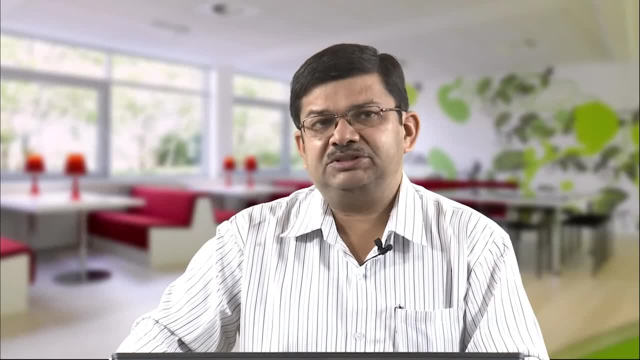 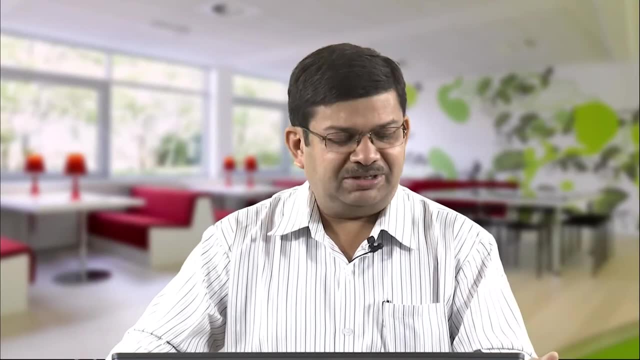 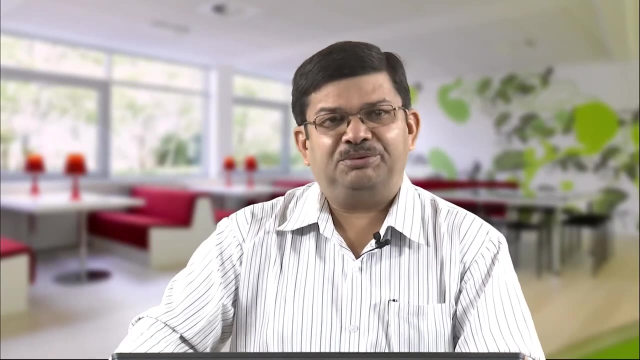 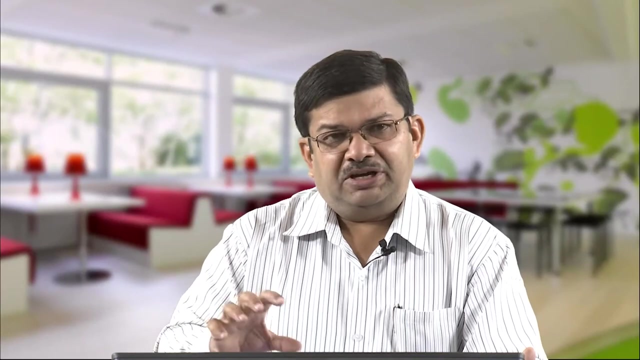 it scales very well from one dimension to three dimensions and the similar construction holds. So these tools get little mathematical tools that we involve. they get little more tedious as the dimensionality of the problem increases but conceptually it remains exactly identical. So we have a differential equation governing differential equation defined over the domain. 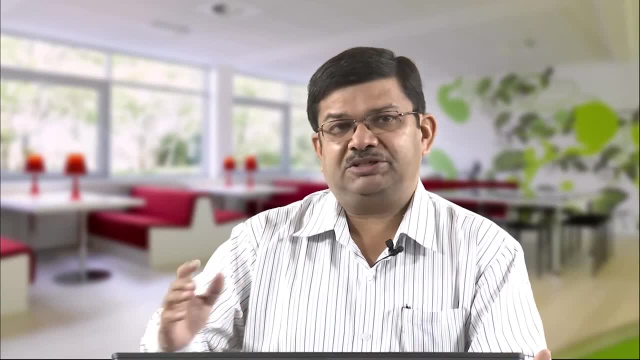 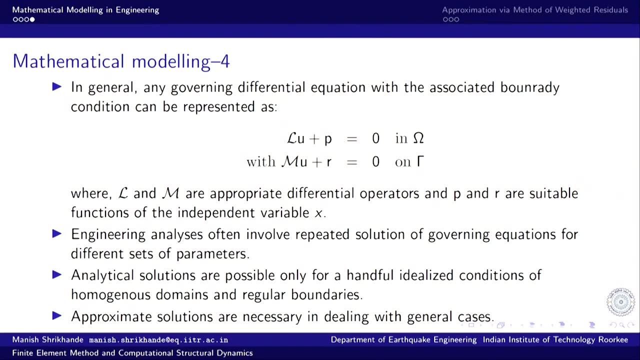 applicable over a certain domain and subjected to certain boundary conditions on the boundary enclosing that domain. Now, engineering analysis often involve repeated solution of governing differential equation. We need to do lots of analysis for different parameters influencing parameters, before we come up with a suitable design or valid design or valid solution to 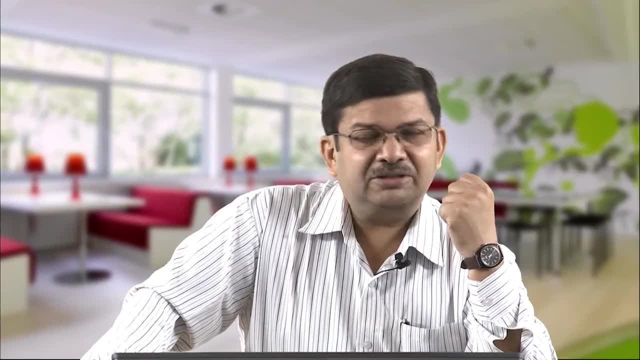 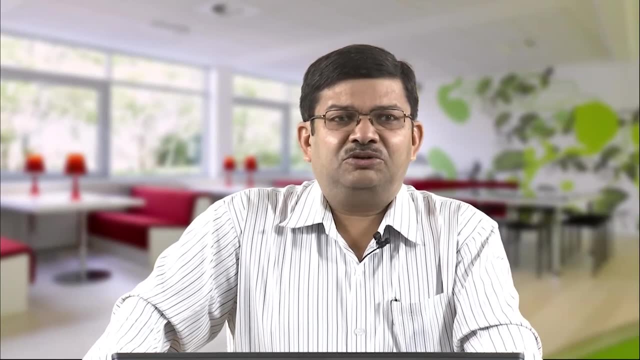 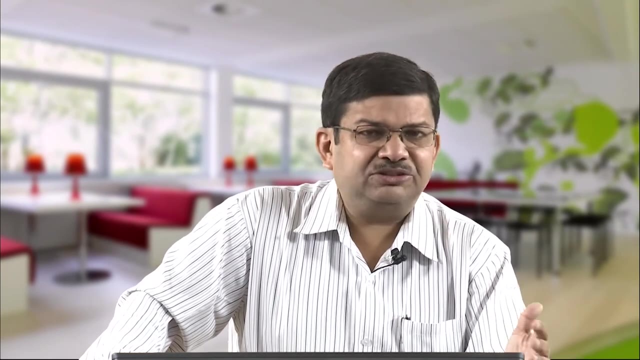 the problem And analytical solutions are only possible for a handful idealized conditions of homogeneous solutions. Now how we are going to apply the laser decreases or conduction. So we have. how do we have to teach the socialоном có 150 states gives about 5 form sickness. you are going. 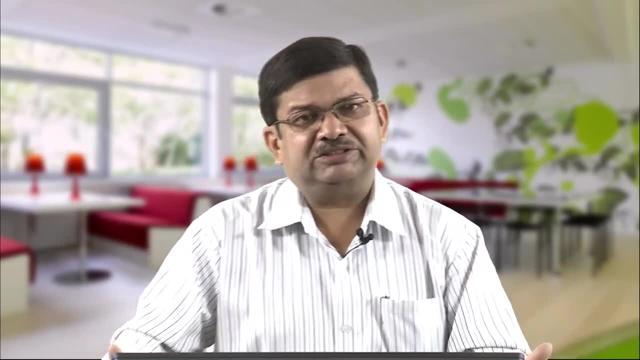 to add somebody to any organized conditions. Well, so the first Owen is the more an average domain, which means in-game, is equal to 0. this dimension is equivalent to 0 becauseீ also has a decentralized function. So this tumor, we take some information. 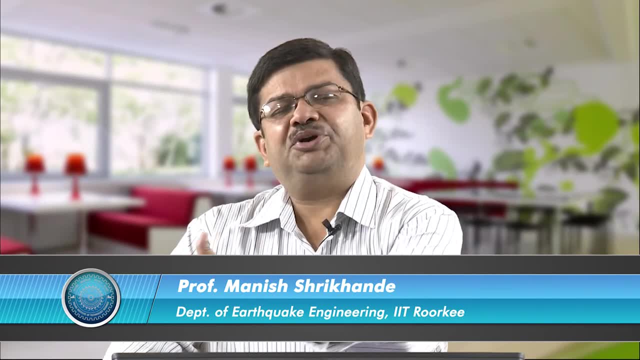 in this domain and, if we look at it, this is the lack of the property覺 Temperature ten 120.. By then the property is less to 0 and this major point is greater than such. so this is very broad. So there, you have a very broad notion here, and these terms are: 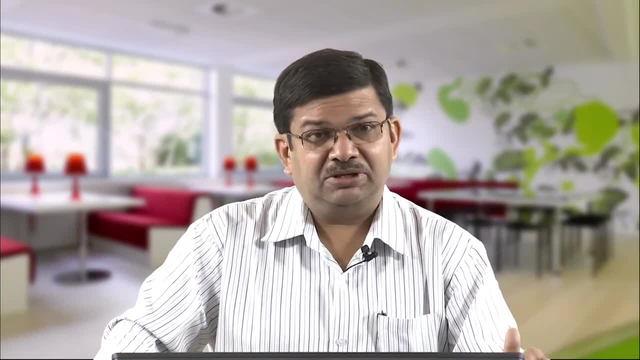 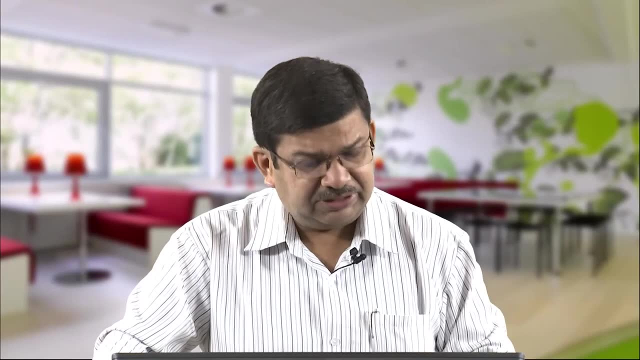 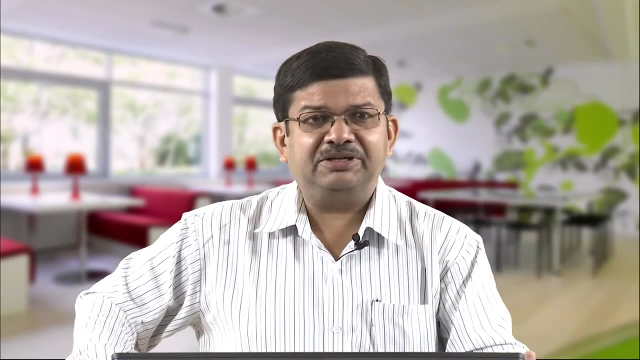 highlighted. If you like, you can go through other dependable выvern征, where these be from crossing line geometrical properties, For example. in this particular situation, the bar problem we discussed. it was we considered a very uniform bar, constant, cross section, constant, same material, If 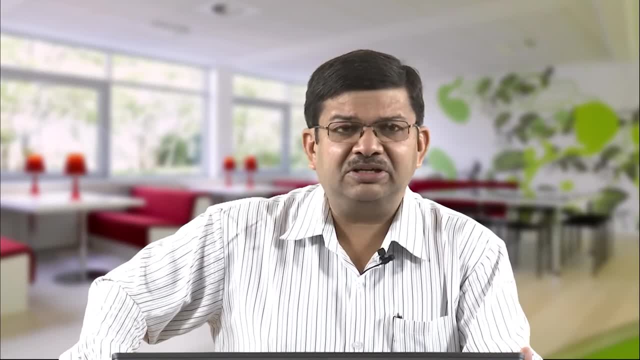 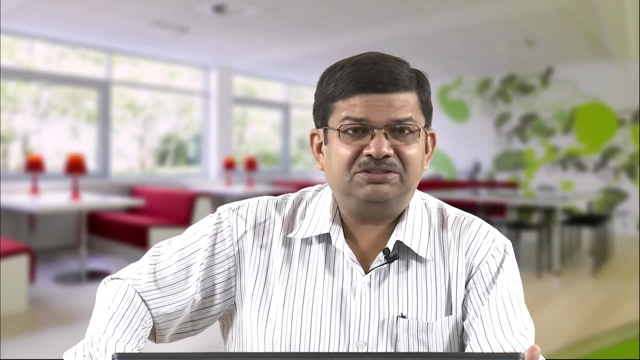 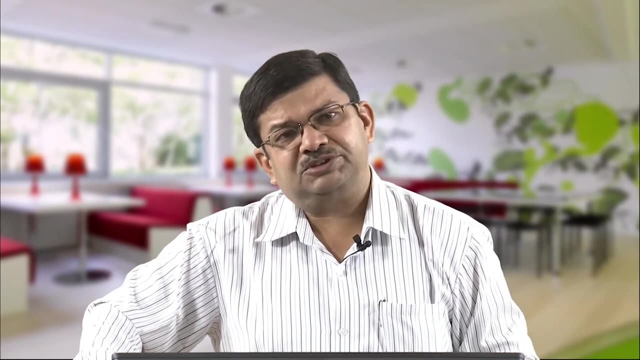 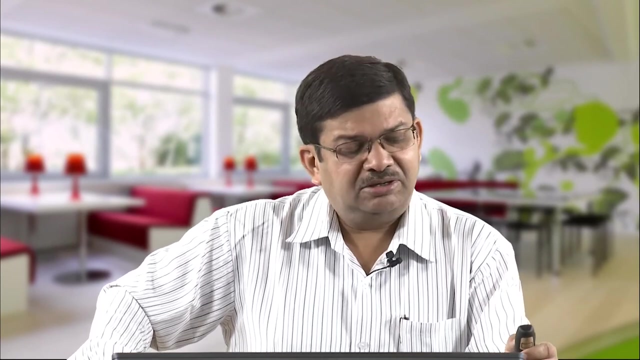 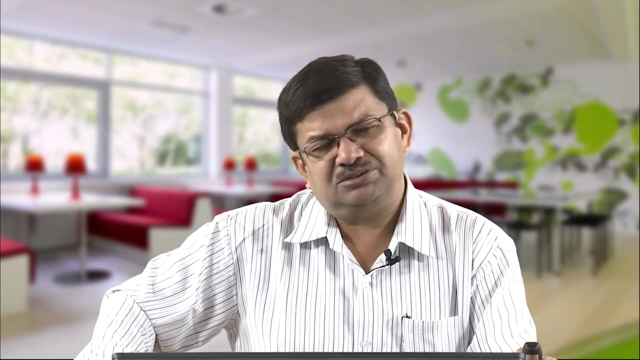 the problem was little different. for example, it was an irregular cross section and the materials were different over different portions- then situation would have been much more difficult and it becomes very difficult to solve analytically this particular kind of difficult or heterogeneous medium. So the domain is no longer homogeneous, So it is still possible if we try and but 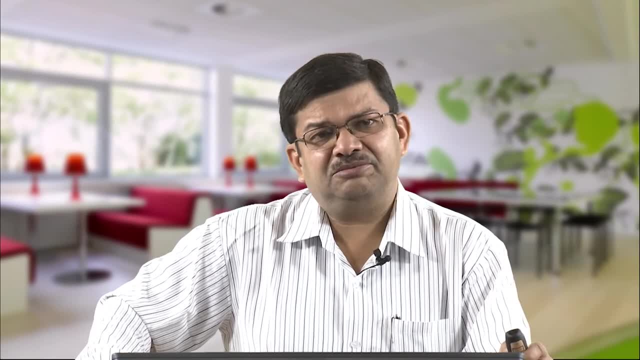 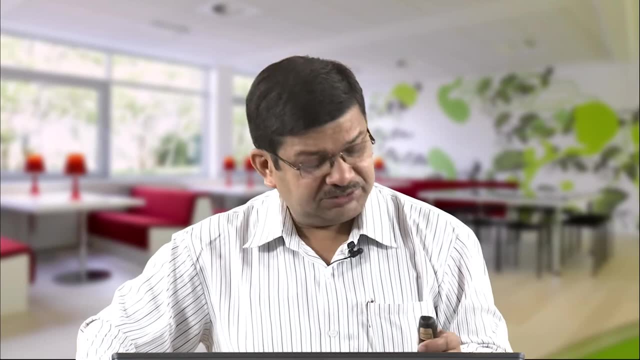 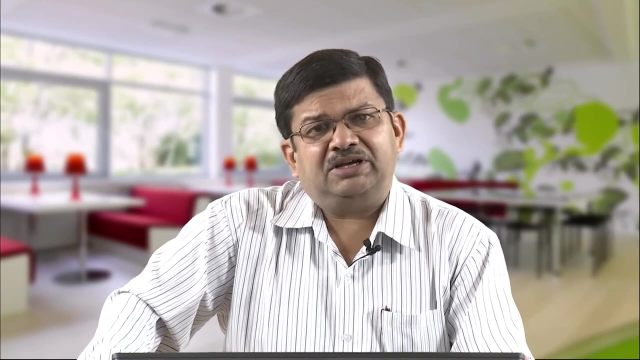 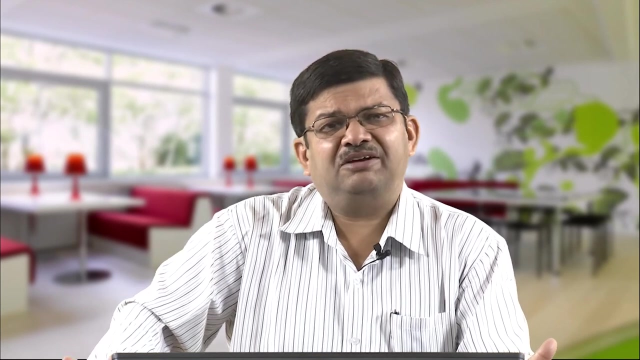 it becomes a little, A lot more tedious and difficult to approach. do it analytically. analytical calculations for you require manual calculations, So for these analytical solutions they are only possible. we can develop analytical solutions only for a handful of idealized conditions of homogeneous domains and regular very well. 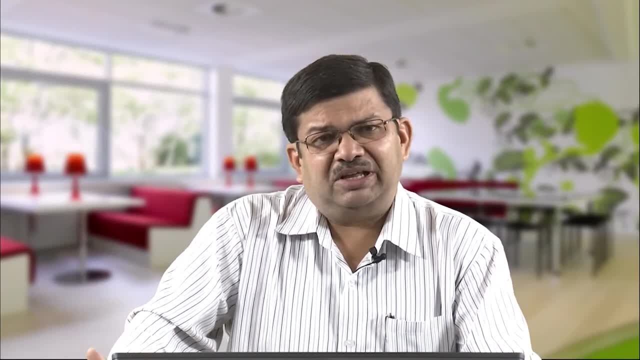 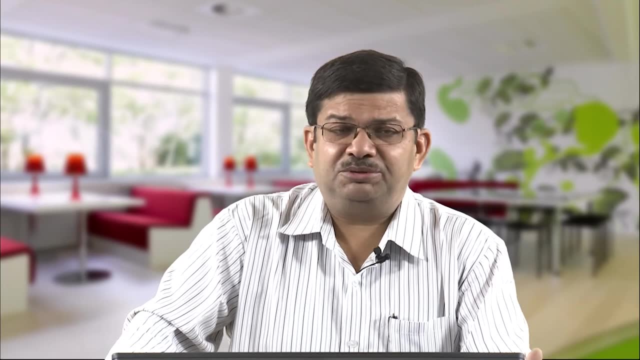 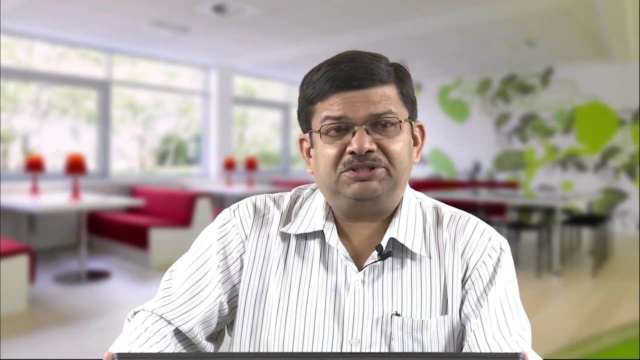 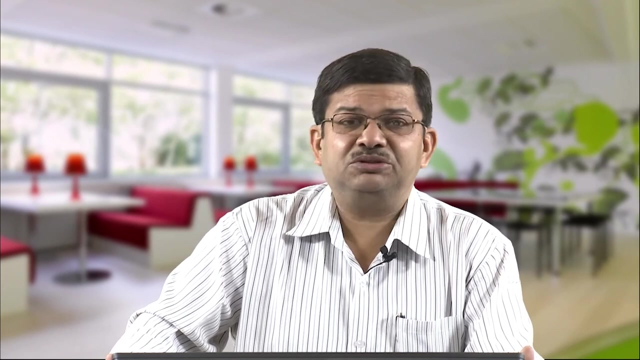 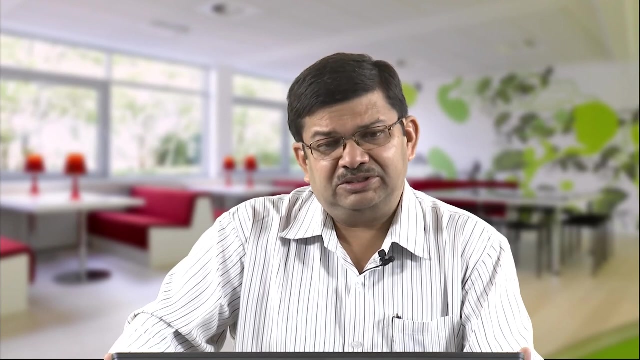 boundaries. The moment any of these idealized conditions are violated, most of the practical problems: they are operating in complex domains using complex materials, So then these analytical solutions are no longer possible. It is not easy to develop analytical solutions, and then approximate solutions are necessary in dealing with such cases, and that is what we will discuss. 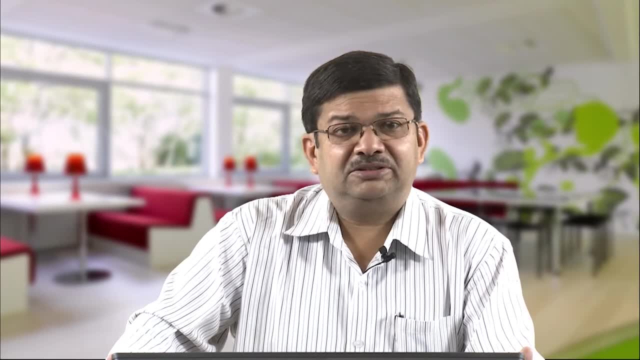 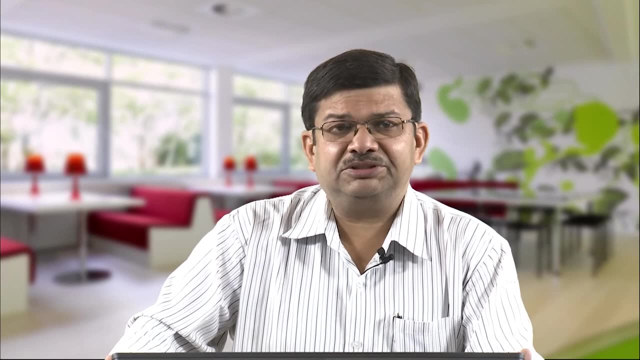 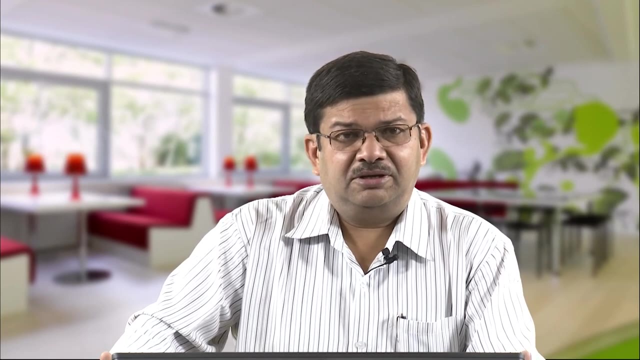 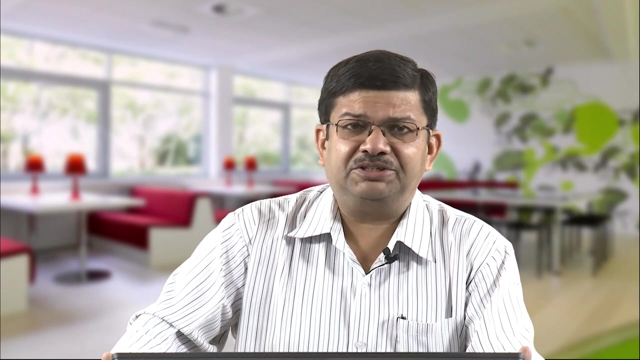 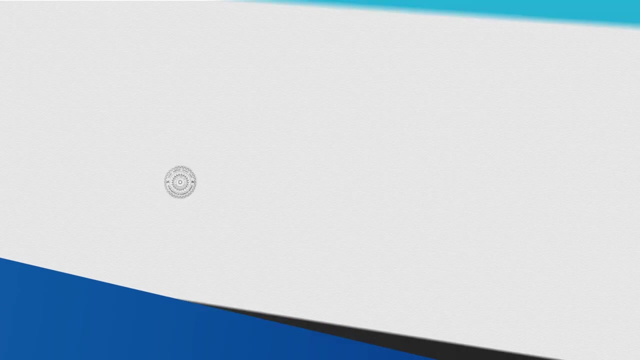 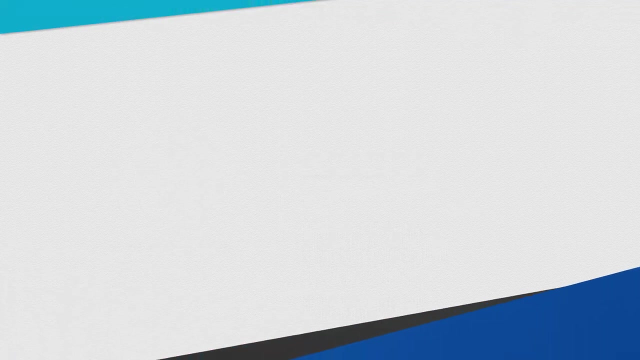 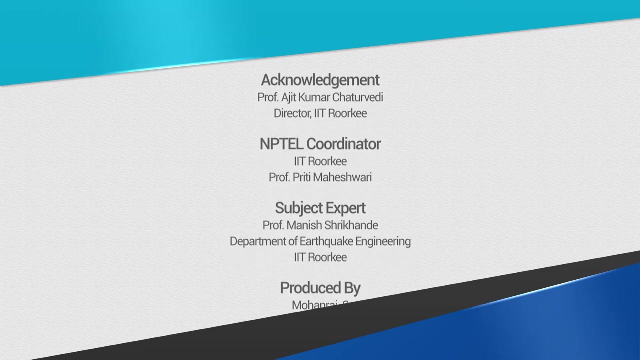 in our next lecture. How do we deal with general solution of partial differential equations using approximate method? approximate solution and that is called method of. So we will discuss method of weighted residuals in our next lecture. Thank you.